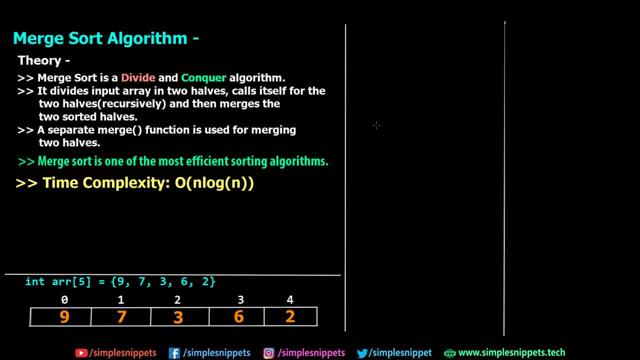 about a little bit of theory and then we will jump into the algorithm. that is the most important part, because that's where we will see how the algorithm works step by step. We will dry run the entire algorithm using diagrams, and that's where you'll understand everything. 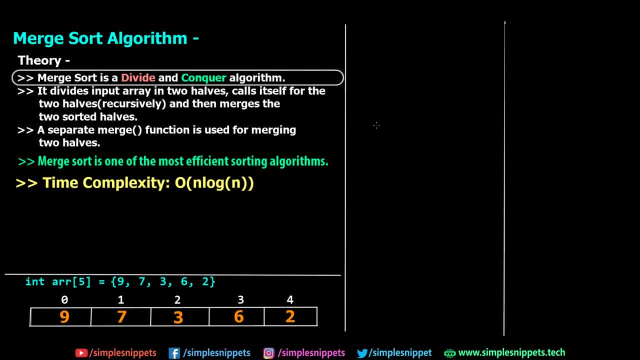 in detail. So let's covered quick theory on this. Merge sort is a divide and conquer algorithm. No, so far as I mentioned, we've covered three algorithms, that is, the selection sort, the insertion sort and the bubble sort- sorting algorithms. but merge sort is pretty. 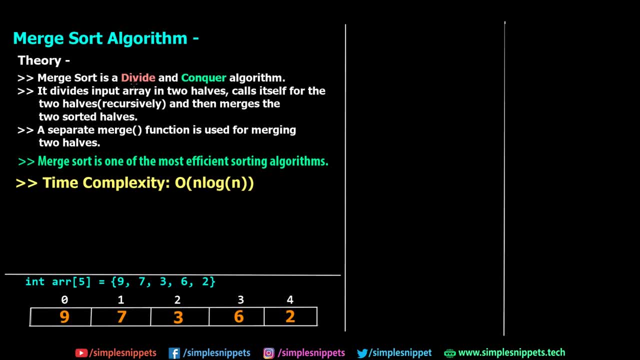 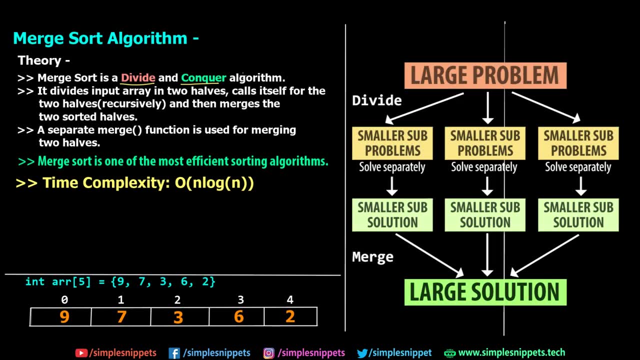 different when it comes to the way it works. Now, merge sort works in a way of divide and conquer methodology. So what is this divide and conquer? So this divide and conquer technique or methodology is a way in algorithms wherein a larger problem is divided into smaller key. 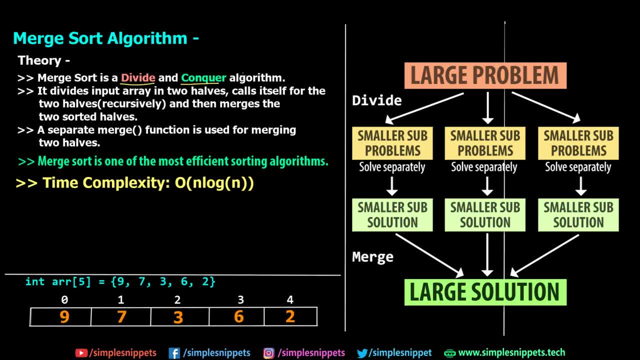 problems or smaller sub-problems, and those smaller sub-problems are easily conquered or easily solved, and then they are clubbed back to get the final result. So what does this help us do? So this helps us in achieving high level of efficiency. and if you see the last point, 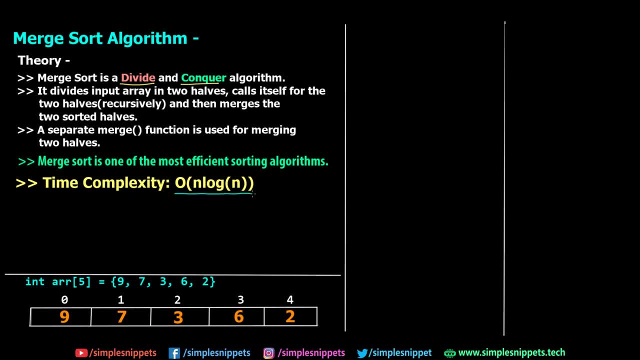 the time complexity of this merge sort sorting is O. Now, if you've seen the first three sorting algorithms in this course, that is, the selection, insertion and bubble sort, the time complexity for those three algorithms was N? square. That is O. By the way, if you don't know what is time complexity, if you do not understand what, 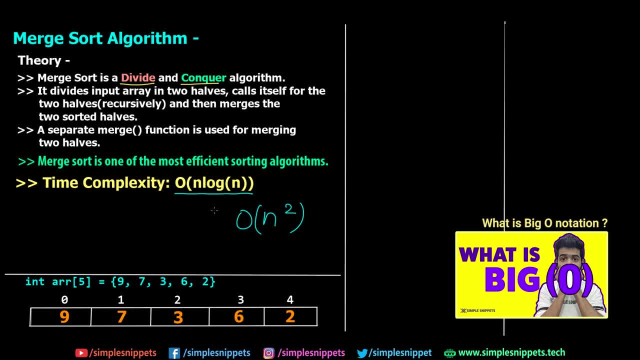 is algorithmic analysis. I have two separate videos in this playlist which talks in detail, and those two videos are also important. you can watch them later on. But what I'm trying to say is those three algorithms, that is, the selection bubble and insertion sort, are very inefficient because of this time complexity. 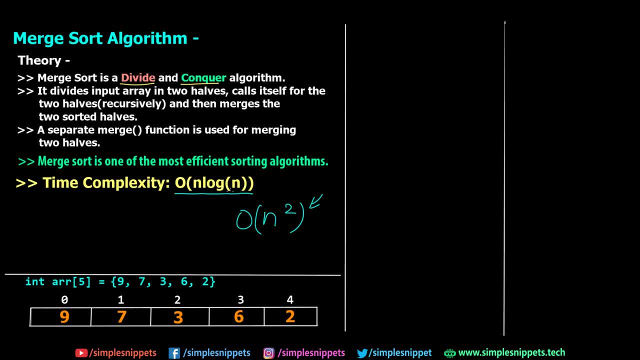 And over here, merge sort has this complexity of N log N, Which is the time complexity of N log N. And over here, merge sort has this complexity of N log N, Which is the time complexity of N log N, Which is supposed to be very efficient compared to O. 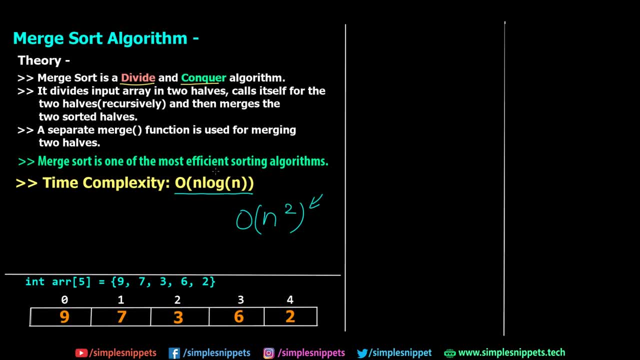 And this divide and conquer methodology is what makes this time complexity much more efficient, and that's why merge sort is one of the most efficient sorting algorithms. Now, merge sort is not the only one which uses divide and conquer methodology. In this tutorial series, if you've seen, we've seen binary search algorithm, which is a searching 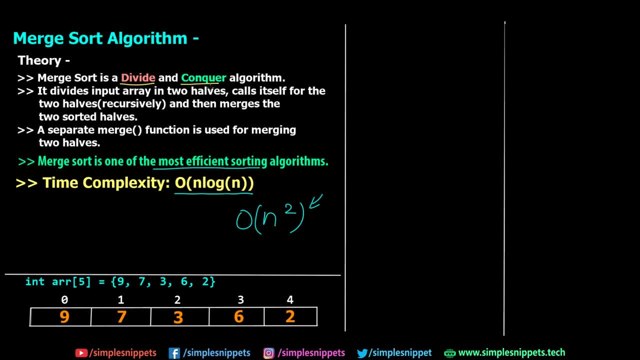 algorithm- not a sorting algorithm, but even binary search uses divide and conquer, because over there we were dividing the entire array, or entire list, into two parts And we were only searching that part where the value that you want to find out fall into that range. 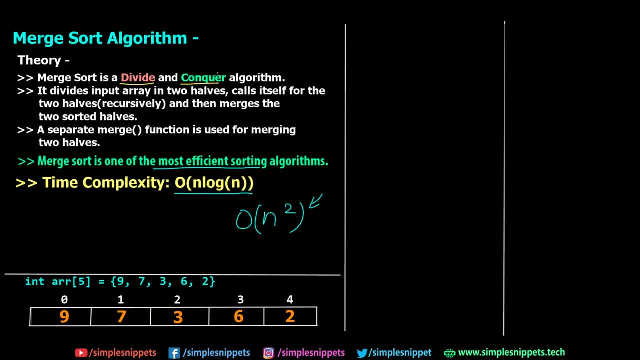 Okay, So the prerequisite was that the array or the list has to be sorted already and only then binary search works. But that was a very efficient algorithm compared to the linear search as well, because it was using the divide and conquer methodology. So what happens in merge sort? 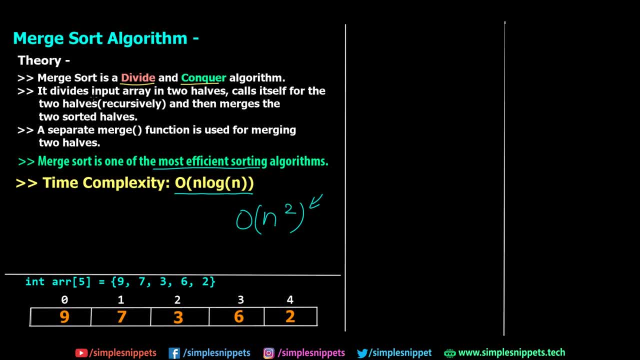 So in in general, theoretically what happens is it divides the input array into two halves and calls itself for the two halves recursively and then merges the two halves. So this point is very important to understand. What is happening here is the merge sort algorithm divides the input array into two halves and 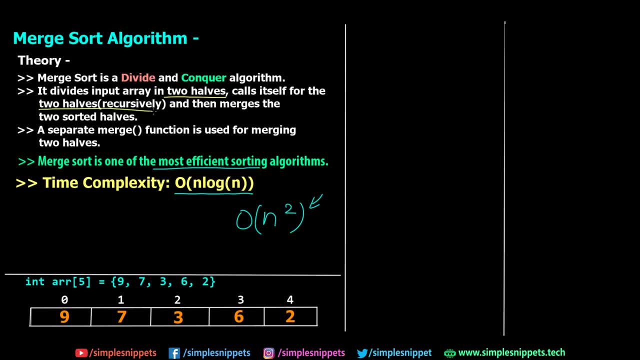 then it calls itself again on the two separate subarrays recursively till we have only one element in the subarray and then it merges the two sorted halves back together. So when we divide an array, let's say we have an array of size four, what this algorithm? 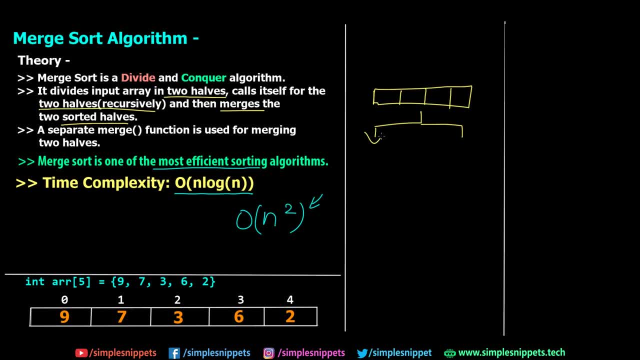 is going to do. It's going to divide it into two halves first, Okay, we get two separate subarrays. Then we are again going to apply merge sort recursively. So this subarray is going to be divided into single single elements or single single sub. 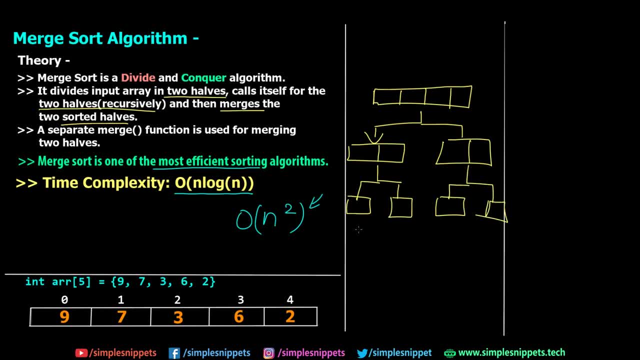 arrays again And ultimately, now obviously we cannot divide this further, right? You cannot divide a subarray having only one element. So now what we will do? we will merge it back again into two and two pieces like this, And then again this is merged back. 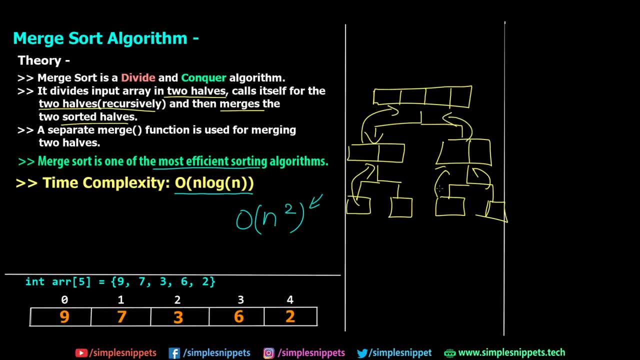 But when we are merging it back again, That is where the sorting happens. okay, So that's the overall concept, or overall working. Of course, we will see in very detail what happens at every call, at every recursive call also, But this is a little bit of diagrammatic sneak peek that I wanted to give you. 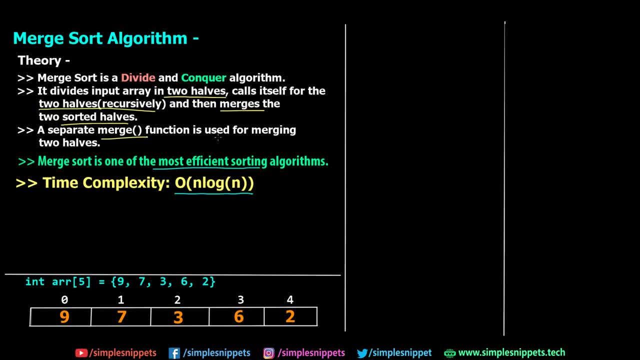 Moving on, there is a separate merge function which is used for merging the two halves. So, as I mentioned, when you are merging the smaller subarrays back again, a separate merge function is called, which is what does the actual sorting. also, So when you are merging it back, you cross check with each other which is the smaller. 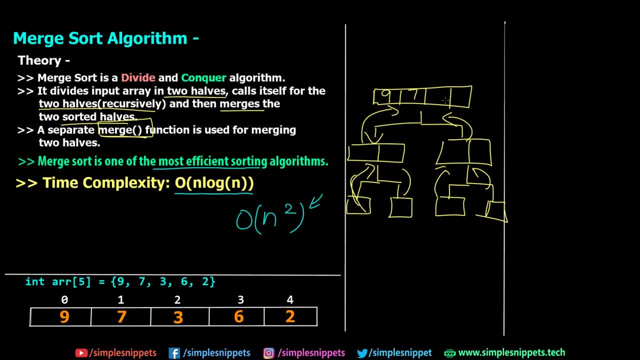 one and appropriately place it. So let's see if it was nine seven. So here's our array right. So we have nine seven, three six. So we have nine seven, three six. again nine seven, three six. 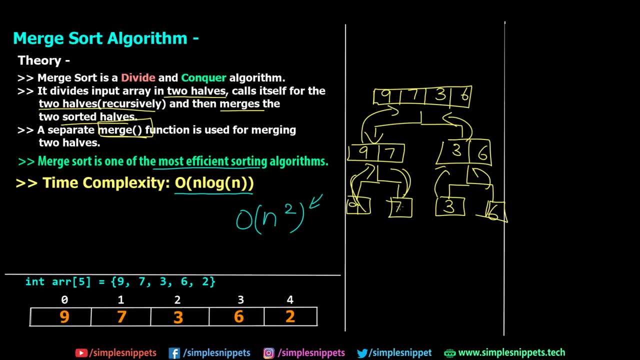 So when you're merging it back again, you can see that nine is greater than seven. So seven is smaller. So when you're merging it, seven should come over here and nine should come over here. So that logic is written in the merge function. 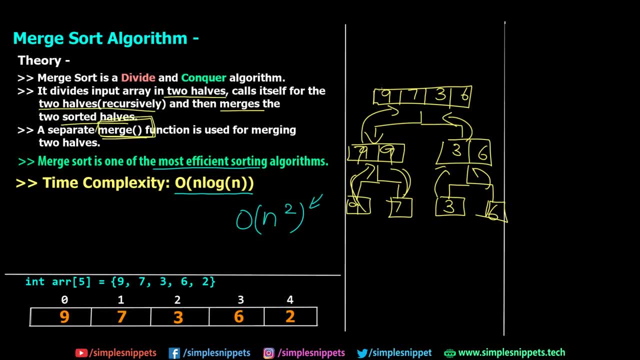 Okay, Okay, So that's the idea. So it's not a big deal, It's just a small detail also, But overall, this is what is happening, Okay, And if you are making some notes, you can note this theory down for your answers. 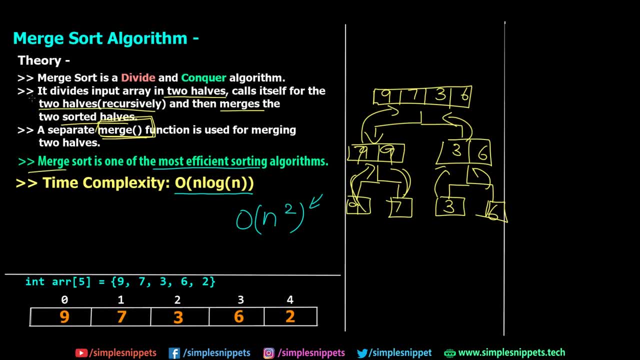 You can note down the time complexity. This is important. This point is important. In fact, everything is important over here. So make a note of it. And now let's actually go ahead and see the four major points, or the three major phases. 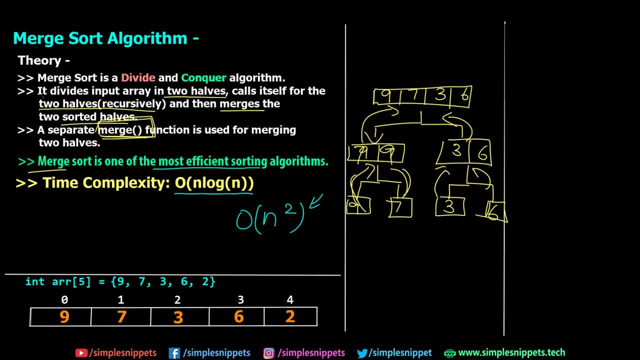 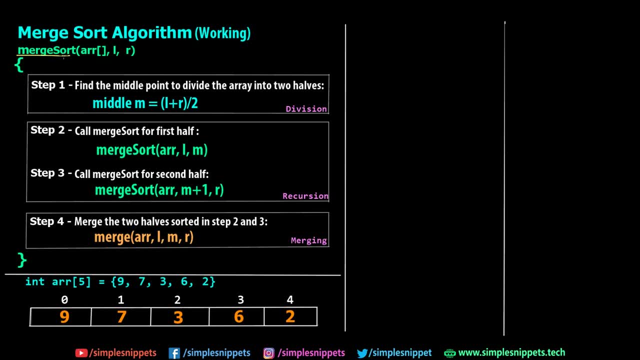 That is the working of the merge sort sorting algorithm, before we actually get into the algorithm. Okay, So, as you can see on the screen, what I've written is: this is the merge sort sorting algorithm. We are supposed to write it in a function format, in a C plus plus function kind of syntax. 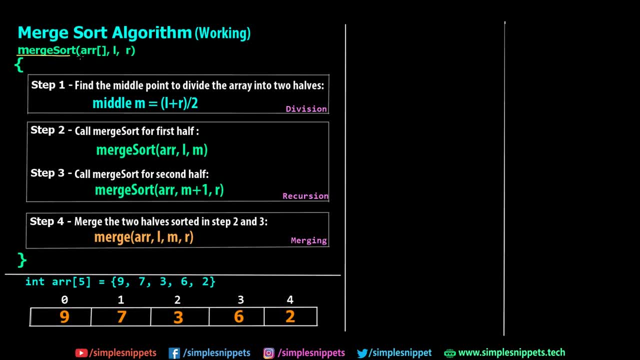 It's not exactly correct, but this is how the merge sort would look like. The first parameter is the array. So our array is going to be a static array of size five. We'll hard code the size for simplicity purpose. This L is called the leftmost index. 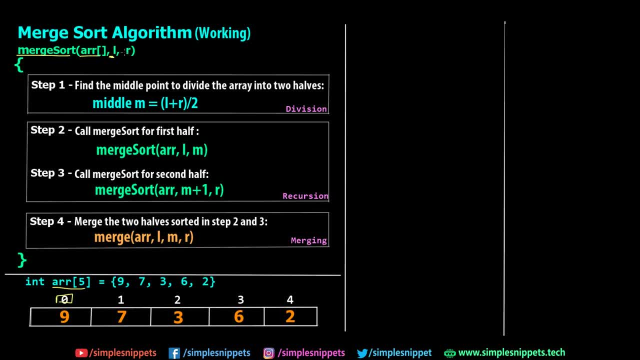 So the left motion index of of course, for the first time, is going to be zero And this R is the right motion index. It can sometimes also be referenced as start and end SNE, And we have different naming conventions. In fact, there is multiple ways to write this algorithm, also when we actually implement. 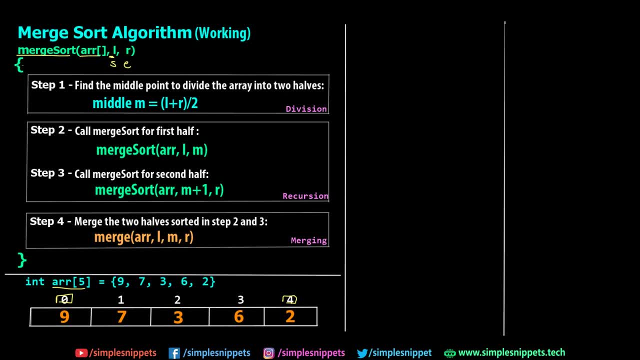 it. But overall these are the three different phases that happen. So inside this algorithm you can see we have step one, step two, step three and step four. step two and three are kind of clubbed together because it's the recursion phase. 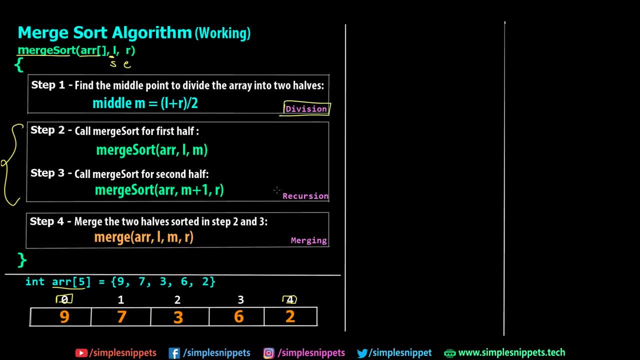 So overall, we have three phases. First is the division phase, The second is where the recursion happens, and the third one is merging it back together. Okay, So step number one. first we have to find the middle point, Obviously to divide the array into two halves, right? 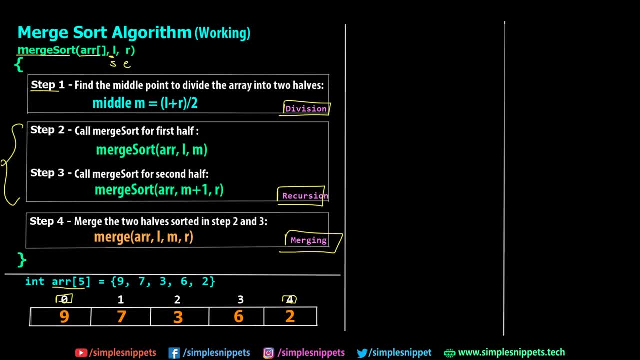 So we have a simple formula: Middle is equal to leftmost index plus rightmost index divided by two. So if you have this array, what would be the midpoint? We have zero plus four divided by two. So four by two it would give us two. 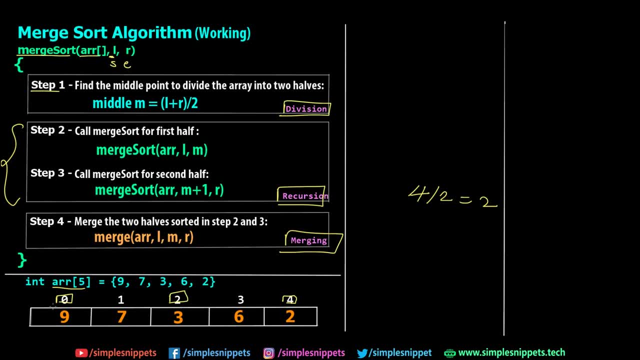 So this would be the midpoint. So this is where we divide. So obviously this is a odd sized array, So we will have two odd subarrays. So this would be the first array and this would be the second subarray. So that's how the division. 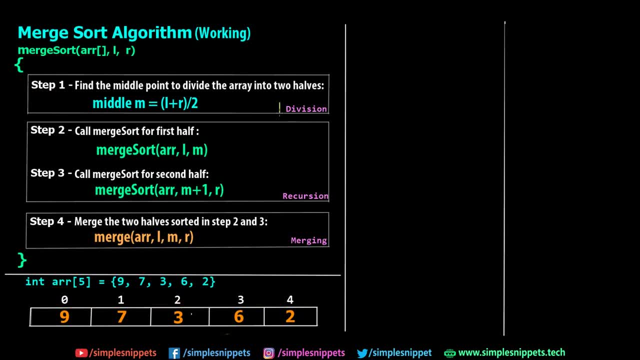 Will happen using this formula. Okay, So now this first step, or first phase of division is. then we've got the midpoint. The second and third step is where we call merge sort, again recursively. So you can see this is the same function, which looks like this: 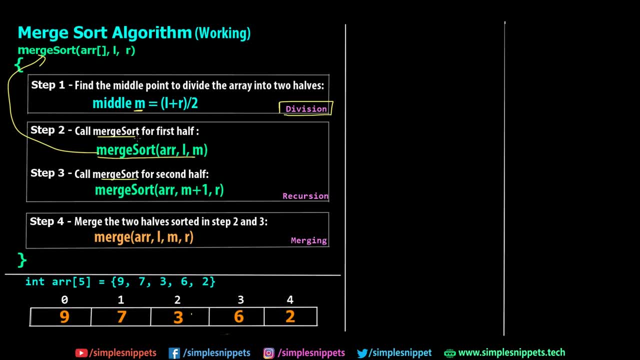 However, only the difference is this merge sort is for the first half, because we've calculated the midpoint. So what we're going to do, we're going to pass the array, We're going to pass the leftmost index as it is, which is L, but the rightmost index. 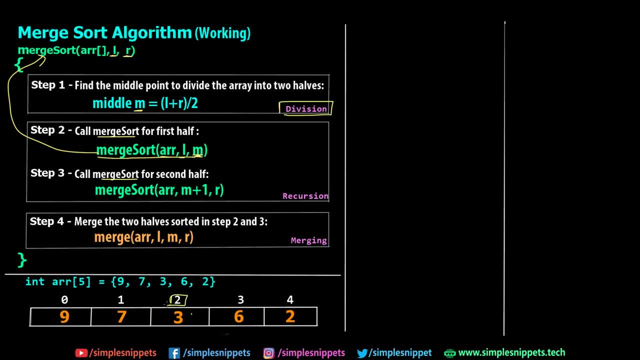 over here is not going to be R, It is going to be M, which is the midpoint that we just found out, And this is for the left subarray. And we again call merge sort recursively, which is for the right subarray also. 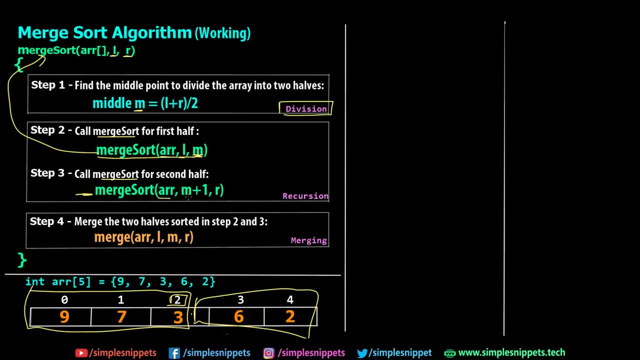 So over here we pass the same array. but now the left index is not going to be L, It's going to be M plus one. So we calculated M as two right. So M plus one would be equal to three. two plus one is three right. 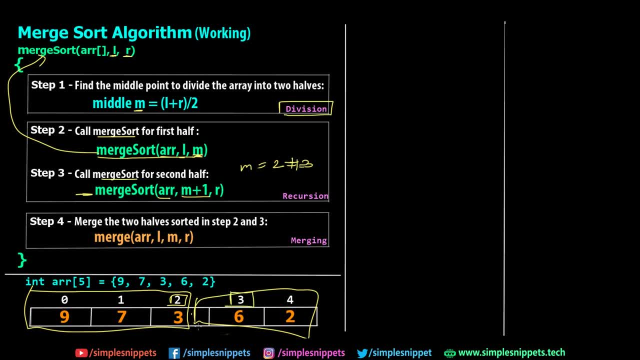 So now this is the starting index, that is left index for the second subarray, and the right index is obviously going to be the same. So so far, so good. So this is the phase. This is where, recursively, the entire array will be divided into smaller subarrays and 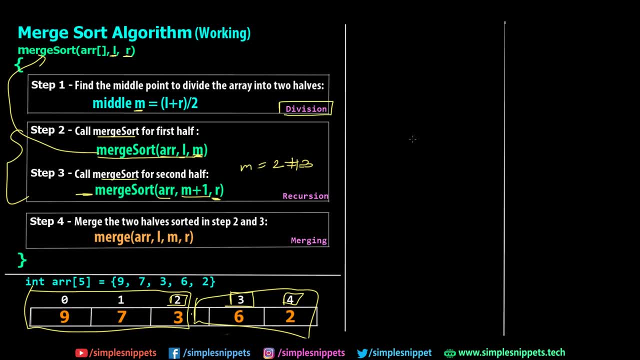 this recursion will keep on continuing till we end up having only one single element in the smaller subarrays. Okay, So there will be a condition, which we will see as we move ahead, where the recursion will stop and it will be like: okay, we cannot divide this entire smaller subarray which? 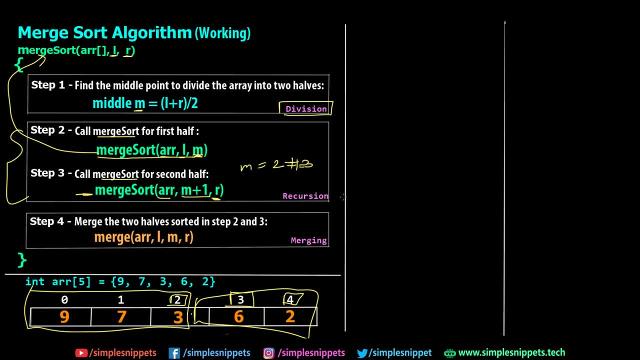 has only one element into further two parts. right, We cannot divide that. So that's where the recursive merging will stop. And lastly, once the division will stop, we will call the merge Merge function. So, as I mentioned, you can see, this merge function is a separate function which will 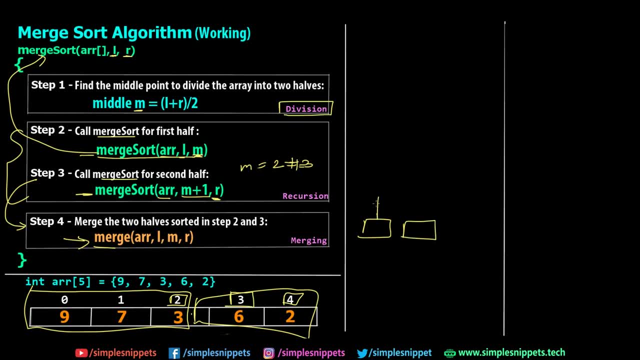 take the smaller subarrays, which are like size one now, once you've completely divided them into smaller chunks, And now we have to combine them back, join them back into larger arrays. So we have to build them from grounds up, And when we are building them- let's say it is nine and seven over here- we have to make 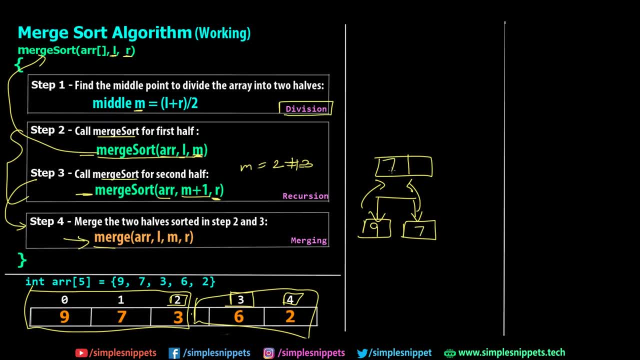 that comparison, depending upon which is smaller: Seven will come over here, Nine will come over here, And the same thing will happen for all the other smaller subarrays when they're combining, And again the intermediate level also. let's say we have seven, nine and three, six over. 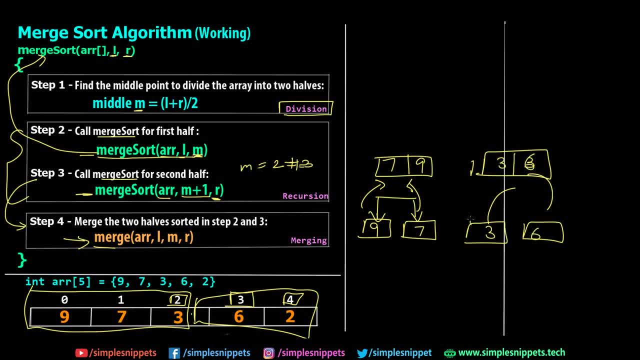 here, right? So? so three and six came over here, but when we are merging them back it will be as it is: three and six, And now we have to merge this also into a larger array of size four. So now again, comparison will happen. 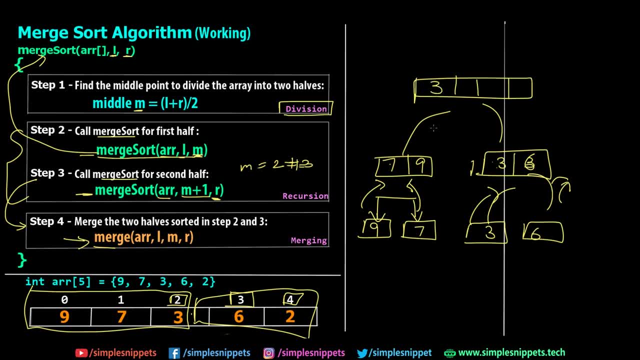 Seven will be compared with three. three is smaller, so three will come over here. Then we are only going to check this one. So now six will be compared with seven. six will come over here, And since we have exhausted this array, then this array will be written as it is: seven. 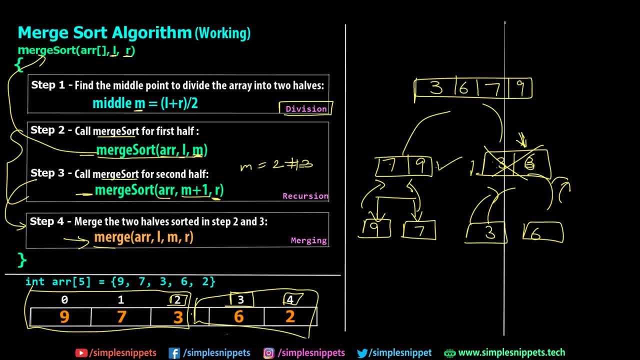 and nine, because this is already sorted. So I'll explain to you this merge logic again properly, when we actually see the algorithm right now. I'm just trying to give you an overview of it, how the merge actually happens. Okay, So three phases, if you're making a note of this: division, recursion, merging. these are: 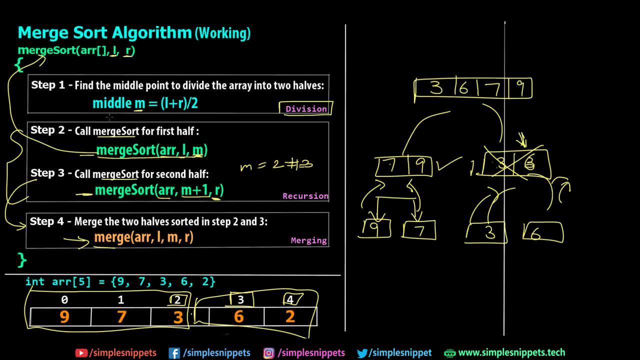 the four broad steps in written in proper English and a little bit of pseudo code kind of language. Okay, You can write it down if you want to actually write an answer, make a theory answer of it. And now that you've got a little bit of overview of what exactly are the broader steps, let's 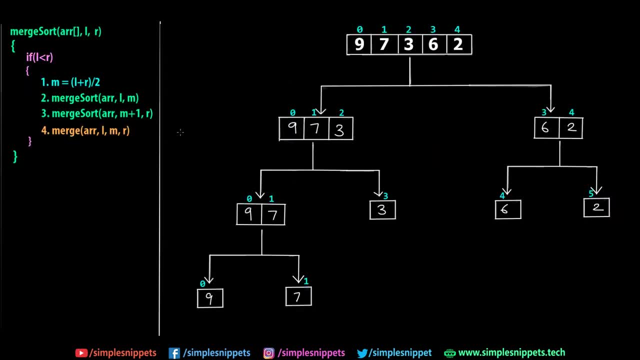 actually see the algorithm in the form of a proper pseudo code. Okay, So as you can see on the screen on the left hand side, we have the same merge sort sorting algorithm in the form of a little bit of pseudo code. So the same four steps that I just explained to you in proper English are now written in. 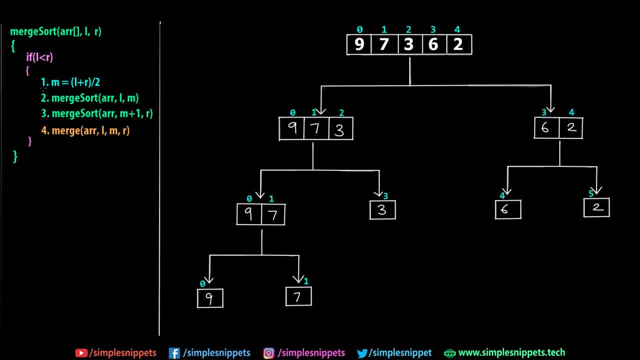 little bit of code format types in a pseudo code format, in stepwise. And we have this. We have this condition, which I will explain: what is exactly happening when we actually run this? And on the right hand side we have this tree structure wherein I'm performing that division. 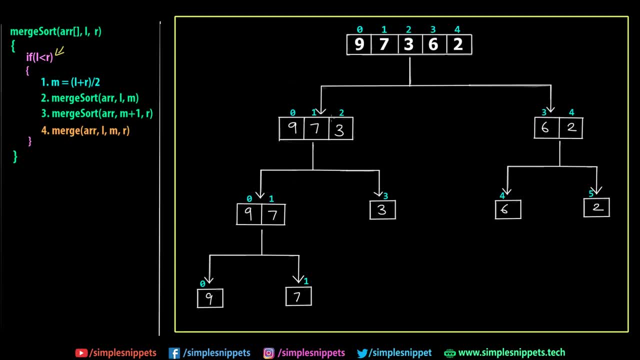 I've already written all the values, but I'll explain how we are attaining or achieving that values. So, to understand this the best way, let's actually try to implement this merge sort on this area. So this is our area, which is of size five. 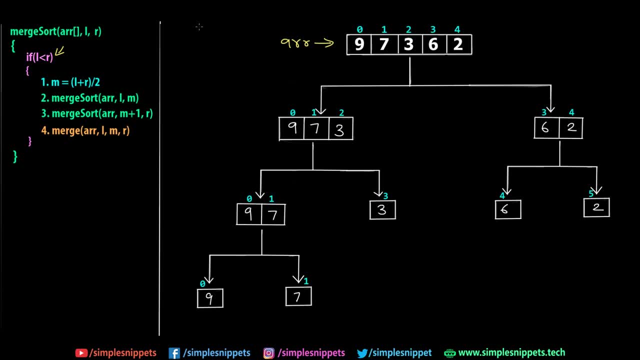 So let's first call merge sort on this area. Okay, Let's give the very first merge sort call. Okay, So, as you can see, I've written merge sort in short form, Ms, Which stands for merge sort, basically, And the call is looking like we are passing the array ARR. 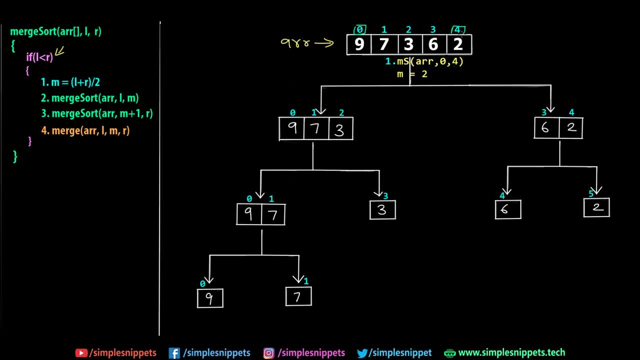 The left index is zero, obviously, And the right index is four. Okay, Now what we do? we go inside this function. Let's dry run it step by step. Okay, Coming over here. The first condition that we check is if L less than R. So what is L over here? 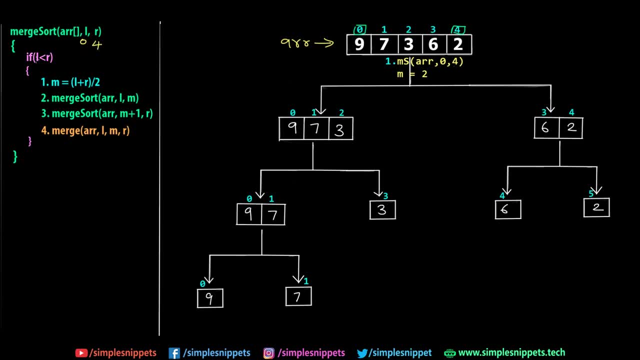 L is zero. What is R? R is four. Now, obviously zero is less than four, which means this condition is true. So this condition actually is for checking whether we are arrived at the smallest sub array, which consists of only one element. 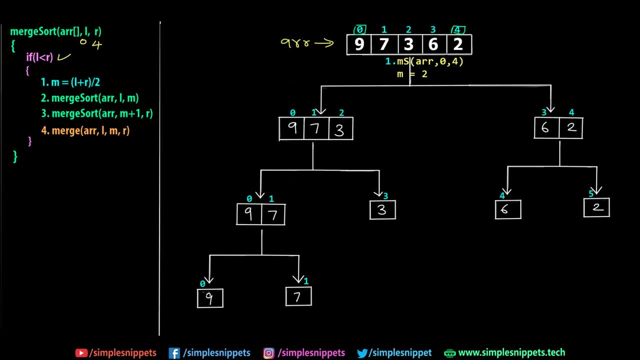 So when we arrive at this, L and R is going to be equal, it's going to be zero, and zero only right. And that's when this condition will become false. So you'll see that when we actually move ahead also. but I'm just trying to tell you in advance. 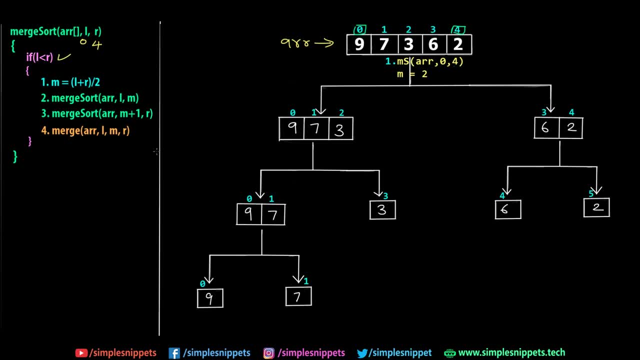 So this condition checks whether we have only one element in the sub array left. If it is only one element, this condition will become false and this recursive nature will stop. But right now zero is less than four, It is true, So hence we go inside this if block. 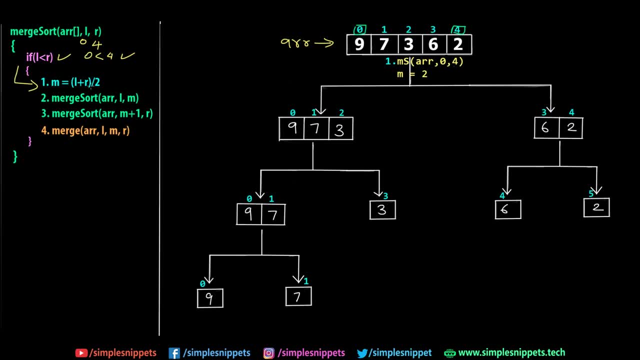 So the first thing that we do is we calculate the midpoint, which is given by L plus R, by two- obviously over here zero- plus four by two, which gives us midpoint of two. So we've calculated two over here, All right. 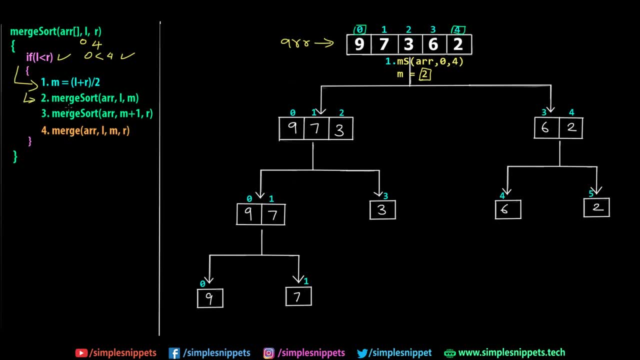 Now what happens is the next step, that is, step number two is where we again call merge sort. So this is a recursive call, right, So this is merge sort, calling merge sort. So first merge sort call was over here. Right Now we are calling second merge sort on the leftmost area. 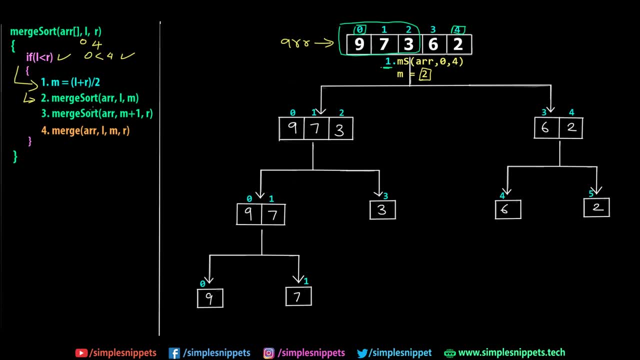 So what is the leftmost area? It is going to be this in this case, because what are the values that we are passing over here? We are passing the area as it is. The L value is passed as it is. L is zero only. 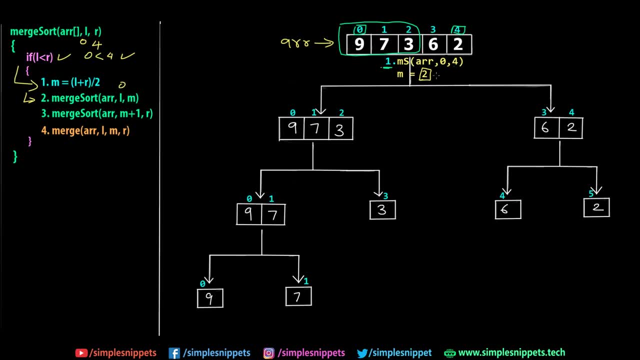 But now for the right value. we are passing the newly calculated midpoint. The midpoint that we calculated is two over here, right? So let me just write it: two over here, and that's what we are passing. So now a second merge sort call is given by the. 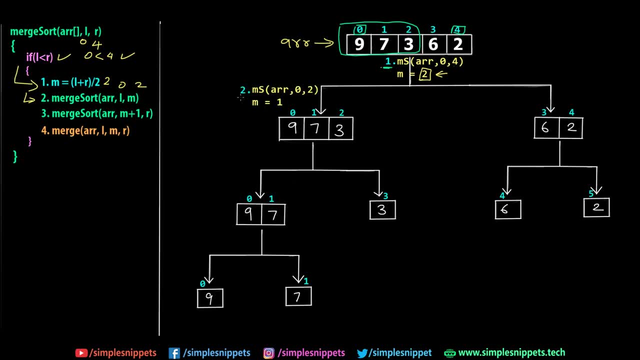 The first merge sort, So let me just show it to you. So this is the second merge sort call which is given for the left side of the sub array. So we divided nine, seven, three and six, two into two sub arrays. 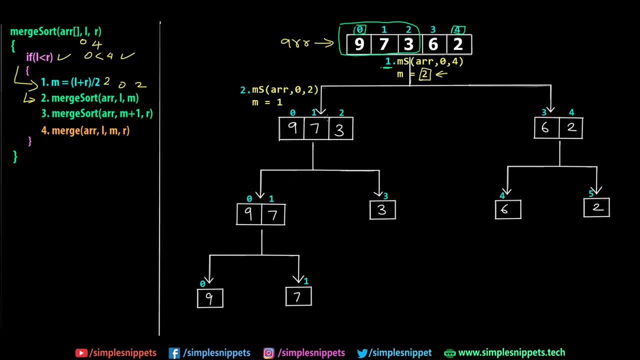 Basically, what we did is we are using the same area only. We are not creating two separate areas. So when we implement this, you'll understand that we are not going to create two separate areas, but we are just applying merge sort on a part of this same area. 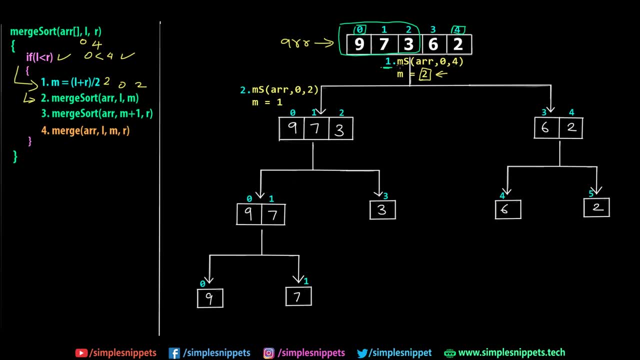 Okay, That's what is actually happening. But now, since this first merge sort has given a call to second merge sort, Okay, This first merge sort will actually go into a pause state, right? So I'll just do a sign of a pause symbol. and it paused at step number two itself because 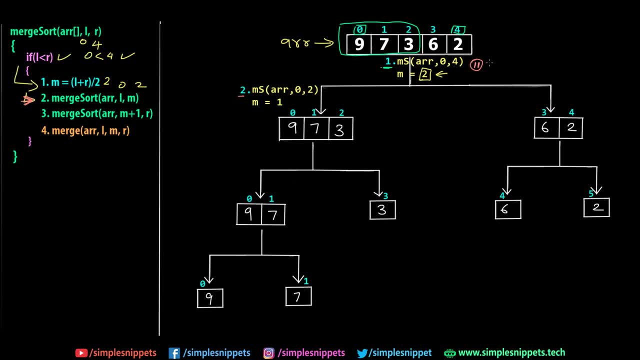 over here. it called second merge sort, So let me just write it over here. It paused at step number two, So remember this, because we're going to come back to this when we actually come outside the recursive functions slowly. So now what has happened is the first merge sort has given a call to second merge sort. 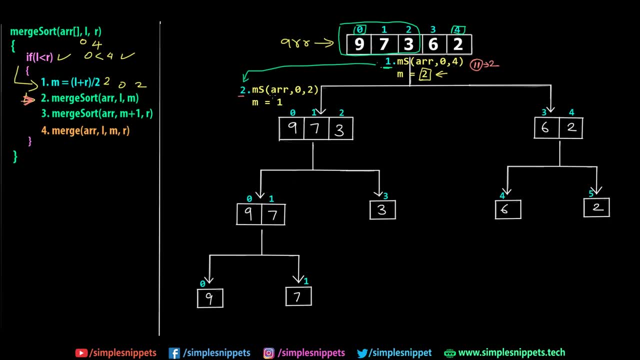 Okay, And second merge sort. we are passing ARR zero and two, So now again we will start this entire process, because first merge sort is paused, So we have to calculate merge sort again for the second call. So let's pass these values again. 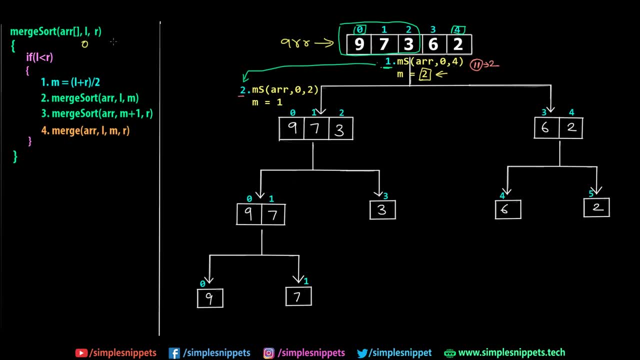 We have the same array. We have passed zero as the leftmost index. The rightmost index this time is two. So again, midpoint is going to be calculated. What is midpoint? L plus R by two? This is zero plus two by two. 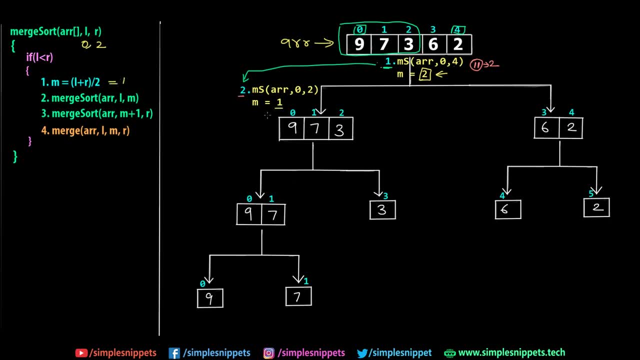 So this time it is going to be one. So here you can see I've written: M equals to one already. So this step is done. for the second merge sort: Now, again we are calling merge sort, and this time it is again on the left side for this: 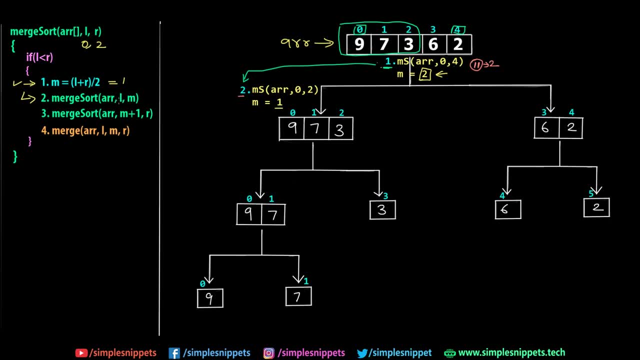 sub array and the values that we are going to pass is the same array. The left is passed as it is, which is L, which is going to be zero only, So zero comma. the M value now is going to be a new midpoint which we just calculated. 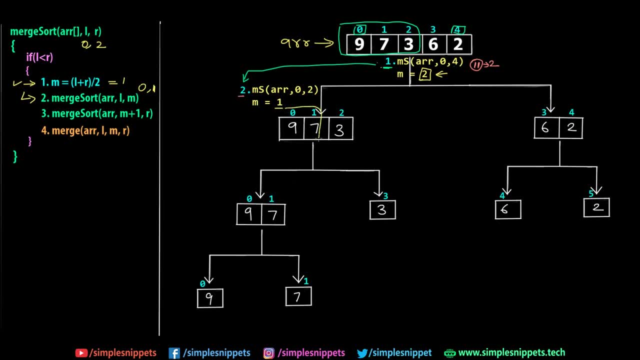 which is one. So we are dividing this array into two parts like this. Okay, So leftmost sub array for this sub array is nine and seven. So that's what is happening over here, which you can see. And now again, since another merge sort call is given by this second merge sort, this merge. 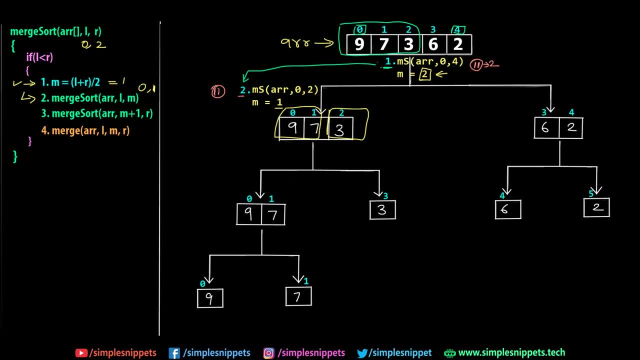 sort again will become paused, So let me just do a pause symbol over here. and this merge sort is again paused at step number two only, So let me write two over here. So first merge sort gave a call, recursive call to second merge sort. 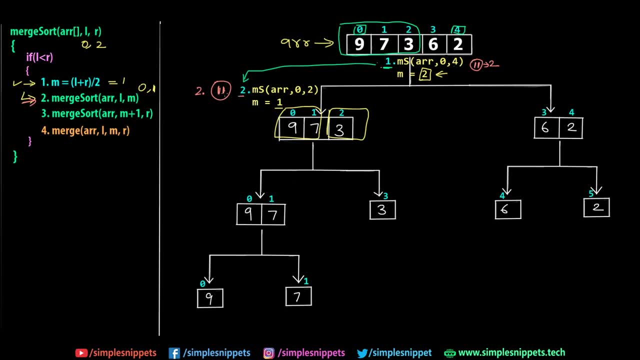 Now, second merge sort is giving a recursive call to the third merge sort and it is going in the pause state. So let's see how the third merge sort looks. And this is how the third merge sort call looks like, because we are applying merge sort. 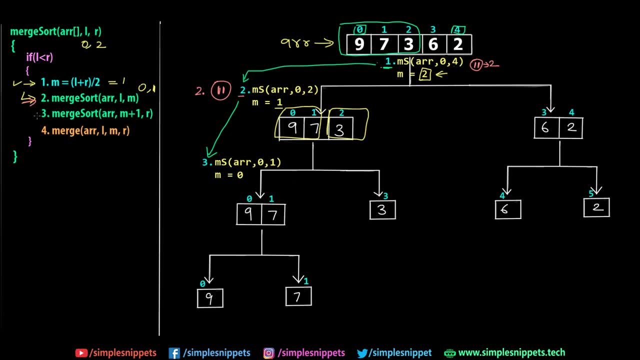 right now on the leftmost side continuously, we are not still going to the third step of any of the merge sort calls, because first all the merge sorts for the leftmost part will happen and that's how the entire algorithm also progresses. So this is like a real world feedback or real world imagination or visualization of what 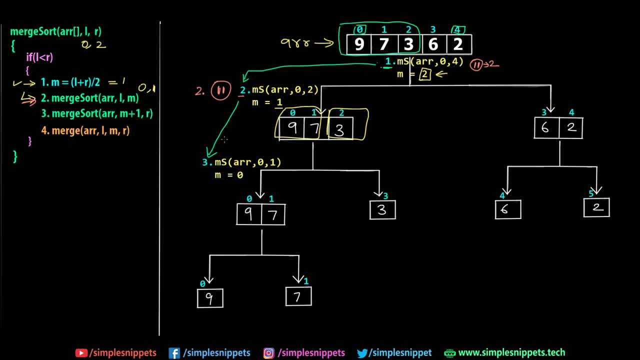 exactly is happening at every step. So now we have passed zero and one, So again merge sort will be executed third time. So third merge sort will start executing, because second is paused over here. So let's execute that Now again. L is passed as zero, R is passed as one. 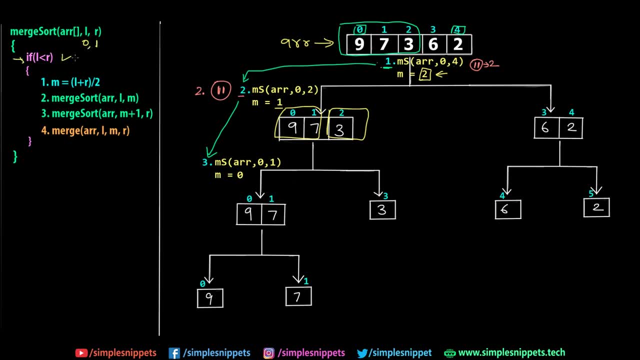 Again, if condition is checked, is zero, less than one. Yes, it is true. So again we will go inside. a new midpoint is calculated. This time it will be zero plus one divided by two, which is going to be one by two, which. 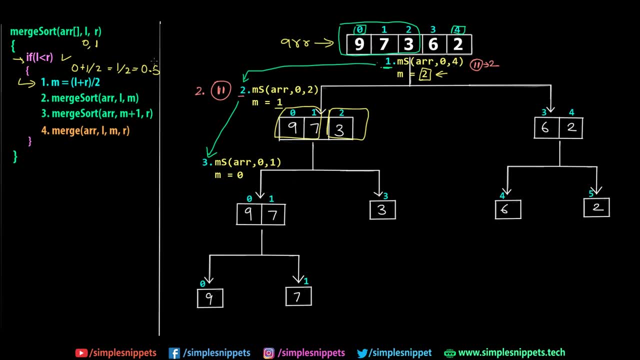 is actually going to be 0.5, but obviously we don't have any index which has 0.5 as the index right, So decimal point indexes. So this 0.5 will be truncated and we will have a new midpoint of zero. 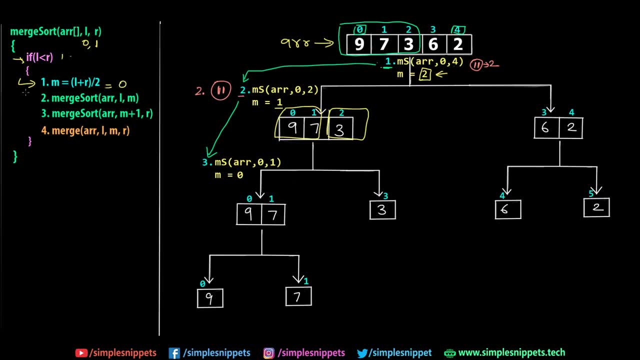 So new midpoint will be equal to zero. Again we will come to step two of the third merge sort, and here again we are giving a recursive call, So you can see this is becoming repetitive. Now array will be passed as it is: The L is going to be zero and M is also going to be zero. 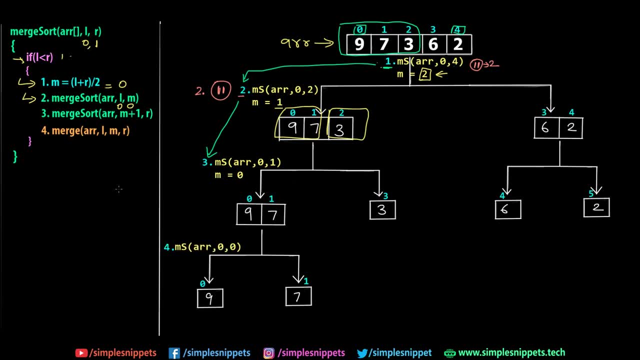 So let's see how the fourth merge sort call looks like. So there you go. we've called a fourth merge sort and this third merge sort has again gone in the pause state Because it has called fourth merge sort, right, So again, third merge sort also paused at second step and third has given a call to fourth. 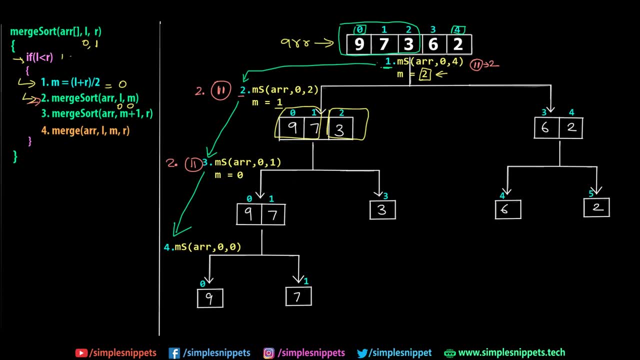 merge sort. So so far you're understanding right. Every merge sort is giving a recursive call to itself and it is going in pause state. The reason why first, second and third are going in pause state is because they have still not finished all the instructions in the function. 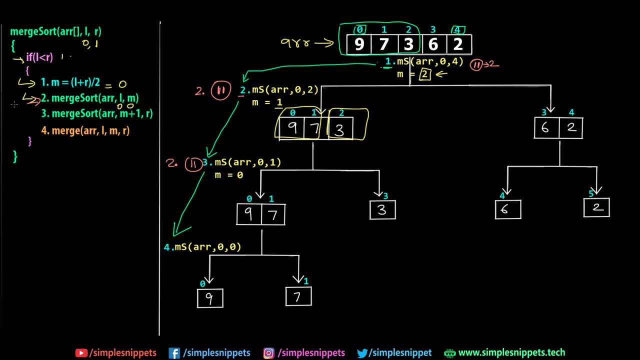 So you can see all the merge sorts that were giving recursive call have been paused at second step only. But you can see we have third and fourth step also, Which means this merge sort, this merge sort, and this merge sort is still incomplete, It still has to execute the third step and fourth step. 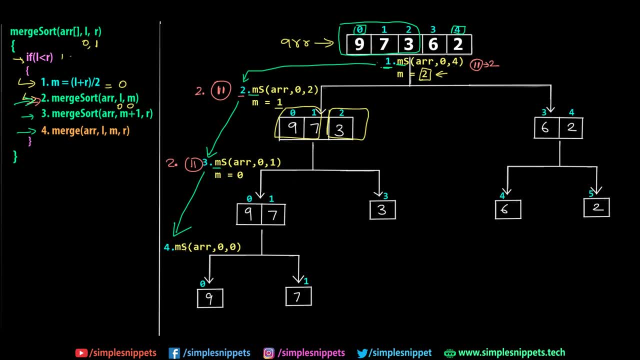 But that will only happen after the last recursive merge sort call completes itself. And now you can see the fourth merge sort call is happening. What we have passed is L as zero and R as also zero, Because midpoint that we calculated was zero. So let's see how this merge sort happens. 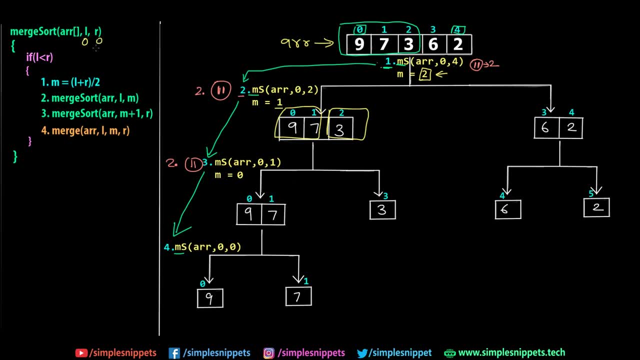 So again, this merge sort will start executing. We are passing L as zero and R as zero And now, if you see, we are checking if L is less than R, L is also zero and R is also zero. Is zero less than zero? 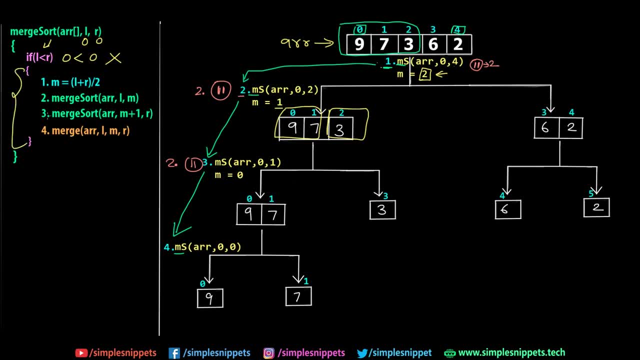 No, this is false. So now this entire if statement will not execute, So that's why we are not calculating a new midpoint right? You can see I have not written M over here, Which means this entire merge sort will complete its execution. 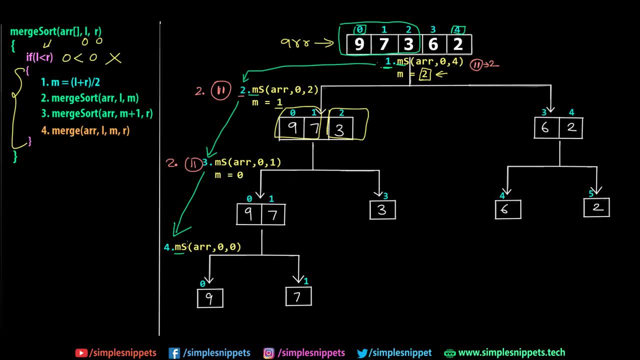 And now it will come back. When I say: come back, where will the fourth merge sort come back To the third merge sort. right, Because third merge sort called fourth merge sort. So when we will come back over here, what will happen? 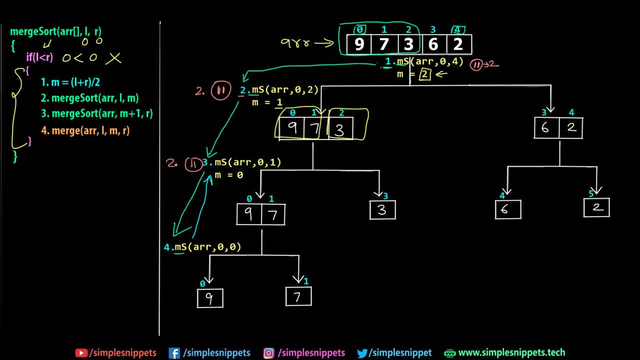 This third merge sort, which was paused. it will resume itself, So let me just erase this sign out. and it had paused at step number two. What was step number two, If you come over here? third merge sort had paused at this state. 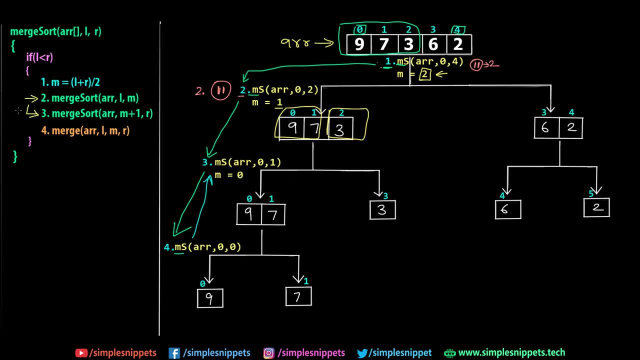 Now this step is done So it will come on the third step. But again at third step you can see we are giving a merge sort call, but this time it is on the right side, or the right most subpart. At third step. 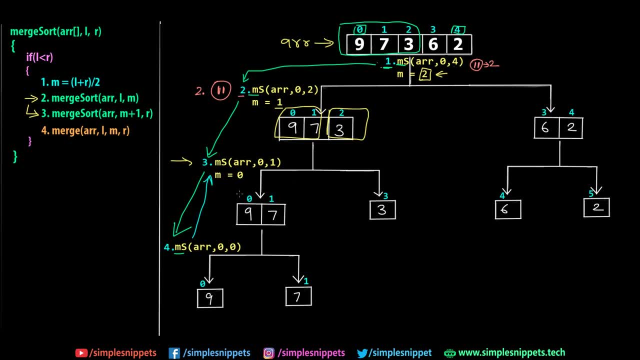 At this level, at the third level. So at third level we divided the array like this: So left sub array has nine and the right sub array has seven. So now we are applying merge sort on the right part because you can see, we are passing the. 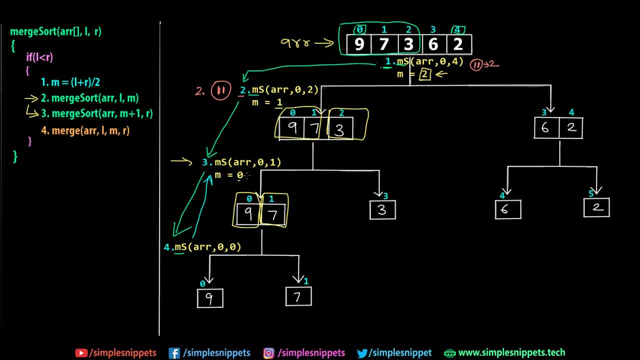 array. We are passing M plus one. What is M plus one? at this level, M is zero. So zero plus one is going to be one. What is the right most value? R is going to be one only at this level. So we are passing one and one. 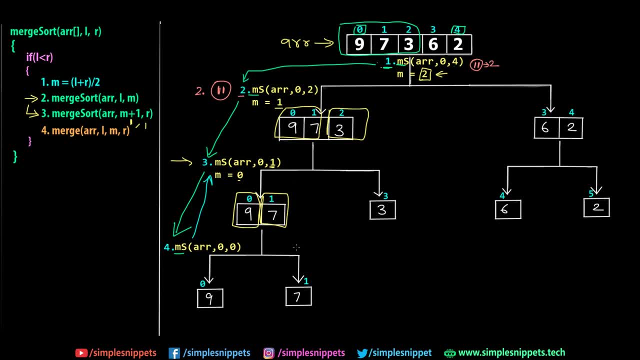 So now a fifth merge sort call is given At this location for the right sub array at this level. So let's see how that looks. So again, this third level merge sort has given a call to a fifth merge sort, So again it will pause, but this time it will pause at step number three. 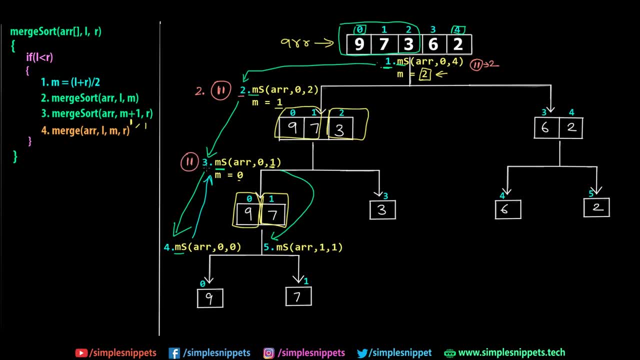 So let me just write that over here Again. the third merge sort, that is number three merge sort, has paused at step number three. This time it is paused at step number three And a fifth merge sort call is given with the values of ARR one and one. 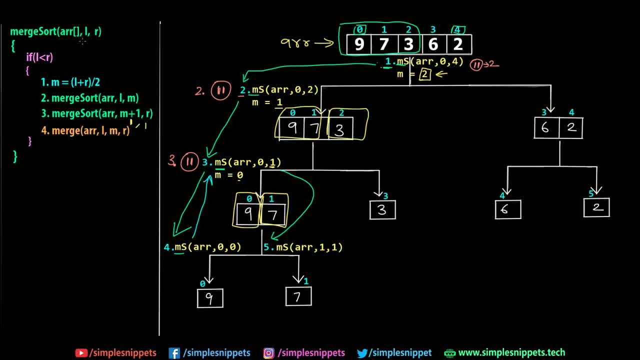 So let's execute this merge sort. So when we pass one and one, obviously this condition again is going to be false, because one is not less than one. So that's why we did not calculate midpoint over here, because this entire if block will not be executed. 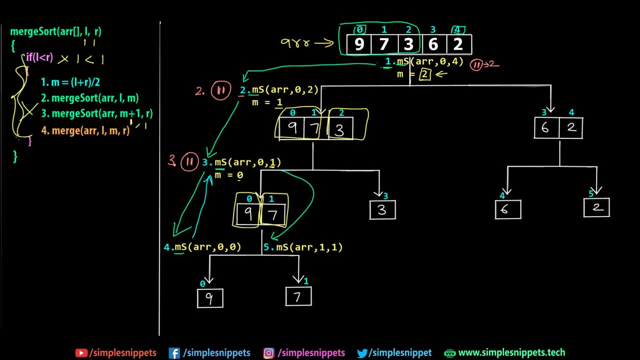 So this complete merge sort will be completed, because we are completely skipping this if block, and that's the only thing we have over here. So we will come outside this merge sort and now we will go back. And where do we go back? We will go back to the calling function. 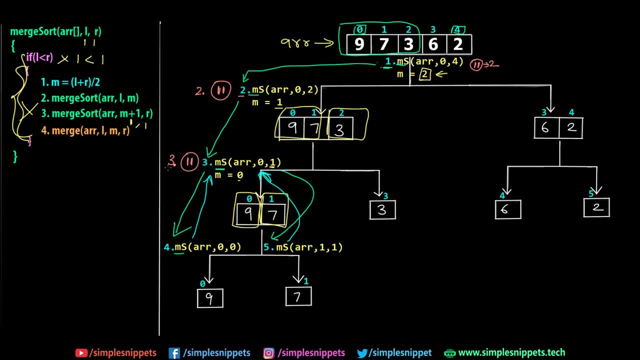 The calling function, This third merge sort call, which was paused at step number three, So now it will again resume from step number three. it's done with step number three, And the last step now is the merge function at this level right. 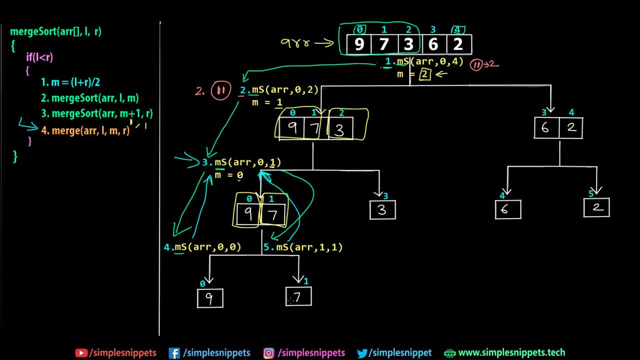 And when we are talking about merge, what we want to do, we want to take these two sub arrays and we have to take them and merge them at this level. But when we are merging it, we also want to compare which one is the smaller one, and we 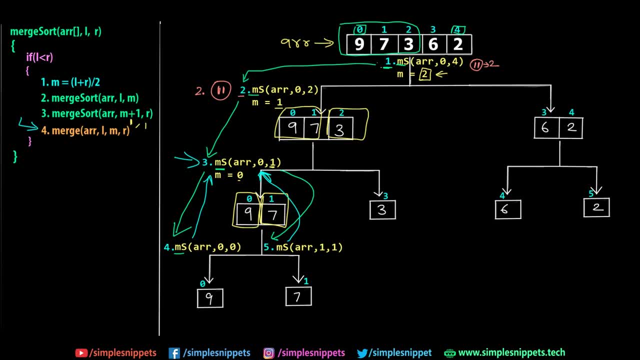 want to sort them accordingly. So what will happen in reality During the merge call or during this fourth step? nine and seven will be compared with each other And, depending upon which one is smaller, we will have seven over here and we will have 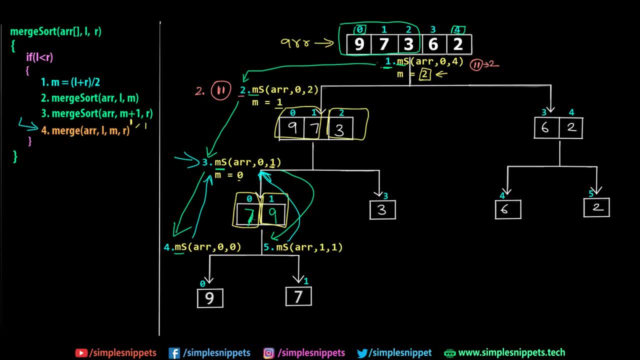 nine over here because seven is smaller than nine, because ultimately, we are using sorting algorithm, We are sorting this in ascending order, right? So seven and nine have been transferred over here. Okay, So we just completely did one complete branch, and if you observe now, what has happened is: 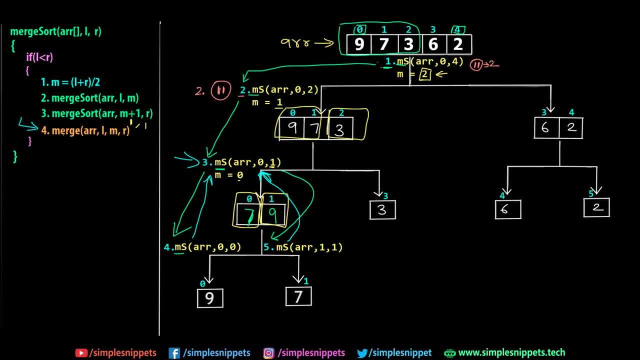 this third merge sort call, Which was doing the step number four of merging, has completed itself. It will come outside this function and this third merge sort will be completely over, right. So let me just erase out everything, because it's become a little cluttered over here. 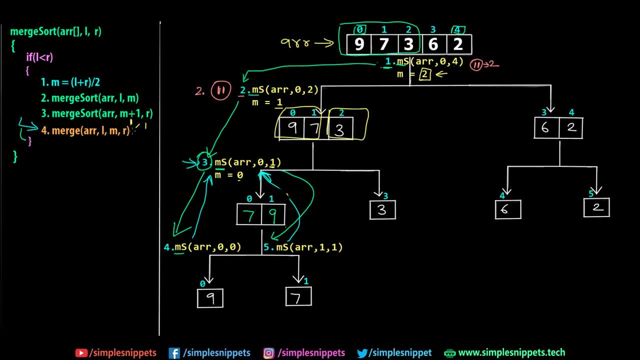 So the third merge sort call, that is, this one has completed all the four steps. But remember that the third merge sort was called by second merge sort. So since third is done, it will go back to the second merge sort, which was you can. 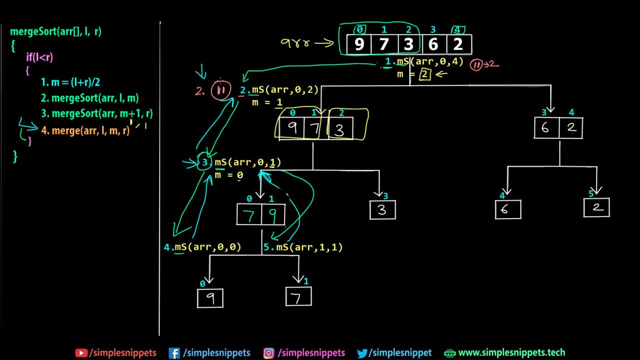 see, is pause that step number two. That's why I've written two over here, right, And there's a pause sign over here. So now we will resume the merge sort at step number two- That is the second merge sort- and resume it from step number three. 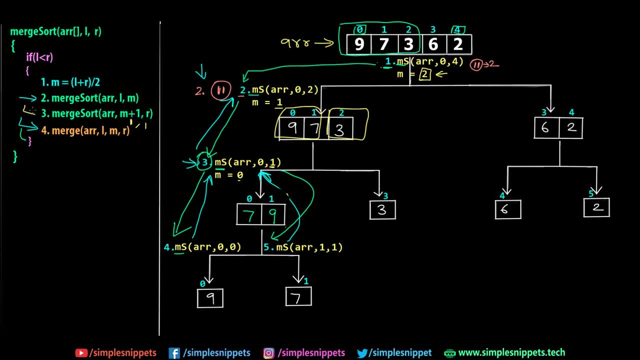 So we had paused it over here. Now we will come one level down and call a merge sort for the right most part at this level. Now, at this level, you can see we have divided nine and seven, which is the left branch which we actually just started. 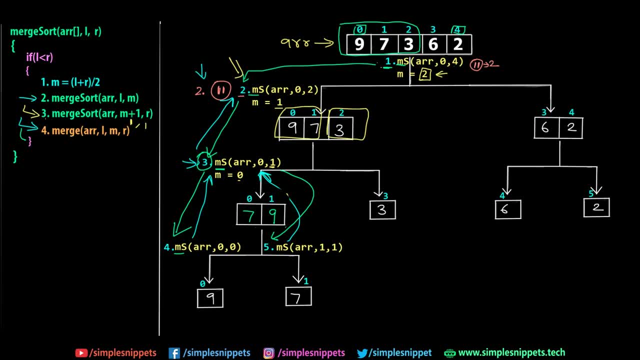 And we also have the right branch over here. So for the right branch we have not yet applied the merge sort. That's why we are applying it at this level. That is, Step number three. So how do we apply merge sort at step number three? for this level, we will pass the same. 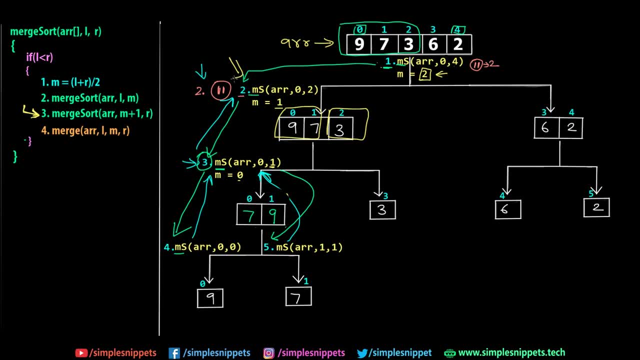 array. We will pass M plus one. What is M over here at this second level? M is one. So we will pass one plus one, which is two. What is R over here at this level? it is also two right. So a sixth merge sort call will be given from the second merge sort. 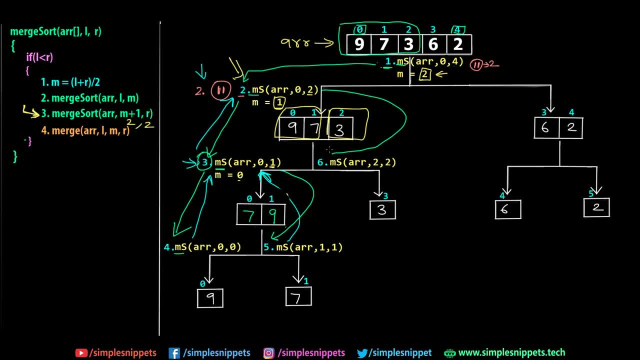 So let's see how that looks. So there you go. You can see this is the sixth merge sort call which is given from second merge sort, right, And again, this will go in a pause state. The second merge sort will go in a pause state, but it will be at the third step. 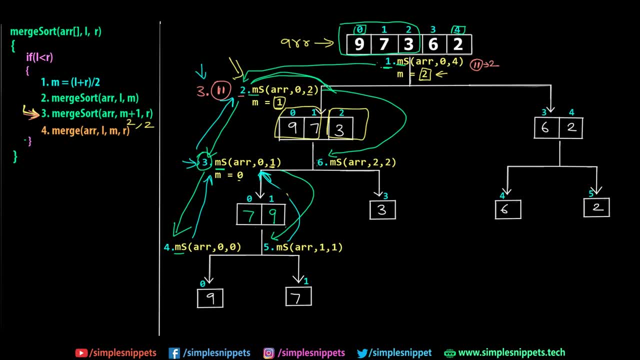 This is where it has paused. now The second merge sort And now the sixth merge sort is executing. again, we are passing two and two. So when we execute this merge sort, we are passing two and two. two is not less than two. 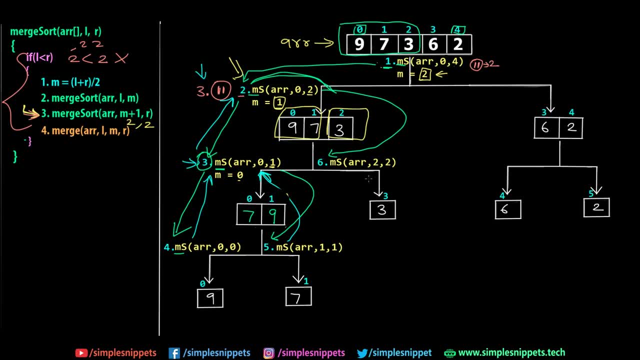 So this entire if block will not be executed over here, So we will directly come back. We will come back to the calling function, which is the second merge sort. I know it is getting a little cluttered, but I hope now you are basically understanding. 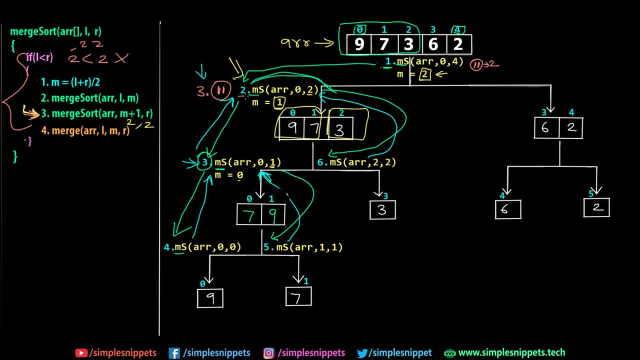 the pattern of recursion that is happening. So we've come back to step number two or second merge sort. Now again, it will resume. So it will resume from step number three only because we had paused it at step number three. This is where we had paused. 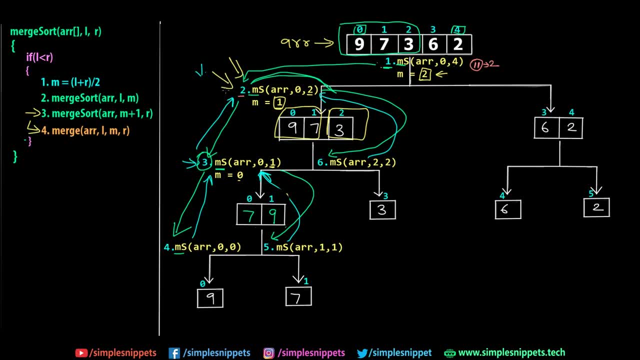 So, lastly, only merge step is left. And at level two, at this level, we have divided nine and seven and three. So we have to merge nine and seven and three. But over here We have already We have divided seven and nine. in the lower steps, 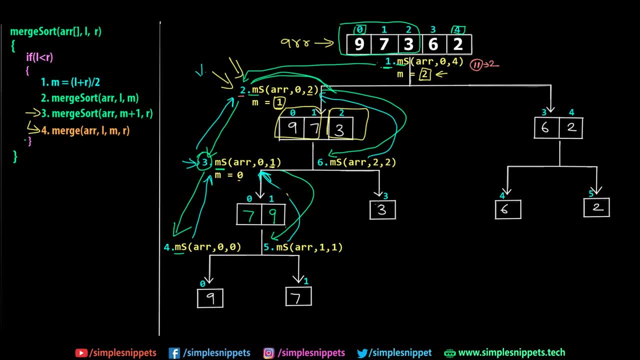 So the merging is actually going to happen between seven, nine and three, right, And the comparison again will happen which one is smaller. So we will check: seven with three is seven less than three. No, three is less than seven. Yes, 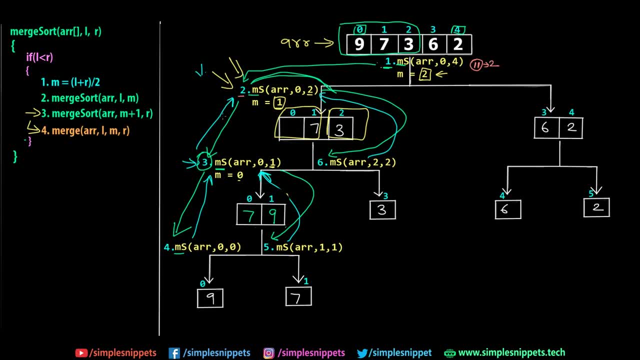 So three will come over here first. So let me write three over here. Of course I will explain this merge, how this merging happens in a minute. right now I'm just giving you an overview. So three will come over here from this and this will be exhausted. 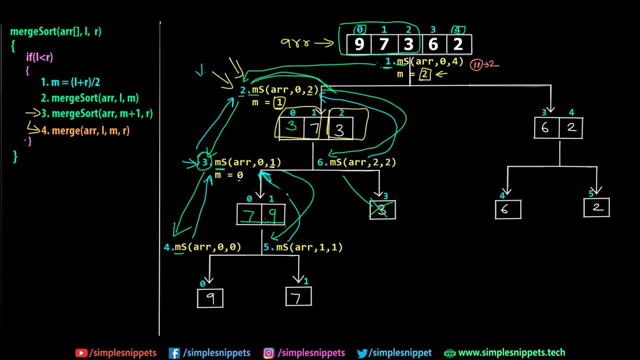 And then seven and nine can be written as it is over here, because it is already sorted right. So let's write that. So seven and nine comes over here, and now you can see that the left part is kind of sorted. We have a sorted sub array. 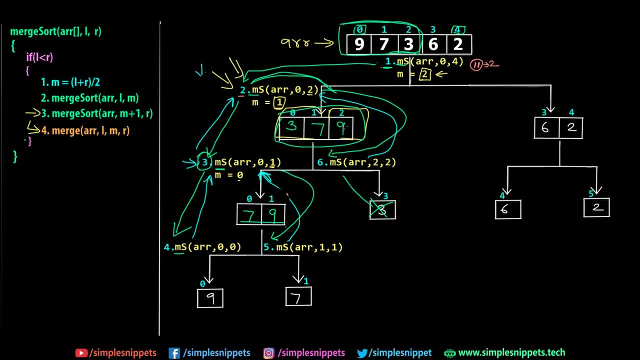 The entire sub branch, that is, this branch is three, seven, nine, which is in a sorted order Now. similarly, the second merge sort will get over because it has executed its fourth instruction. We were at this level who had called the second level. 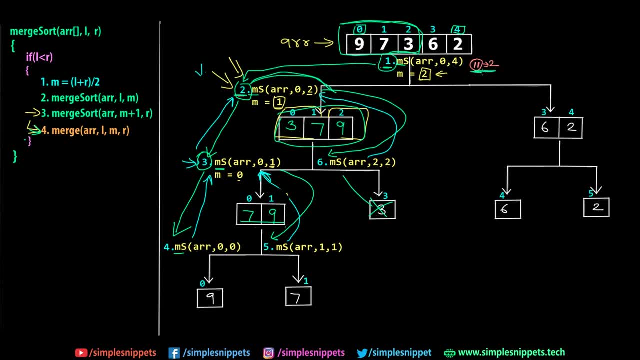 The first Merge sort, which has also been paused at step number two, right. So now second will go back to step number one, That is the very first merge sort. Where was the first merge sort? paused at step number two, which is this step: 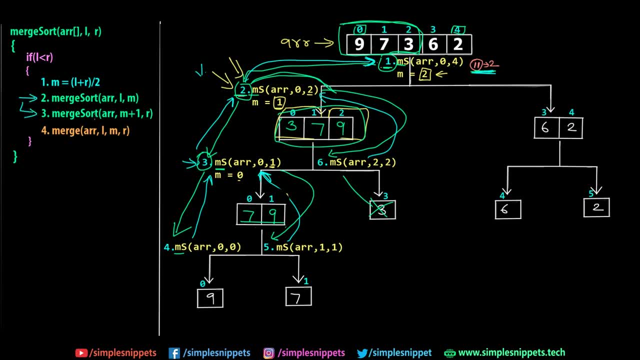 So now it will move to step number three, and step number three is applying merge sort on the right side, which is the right side. at this level. We have six and two, which is this side. So now a seventh merge sort call is going to happen, because sixth was over here. 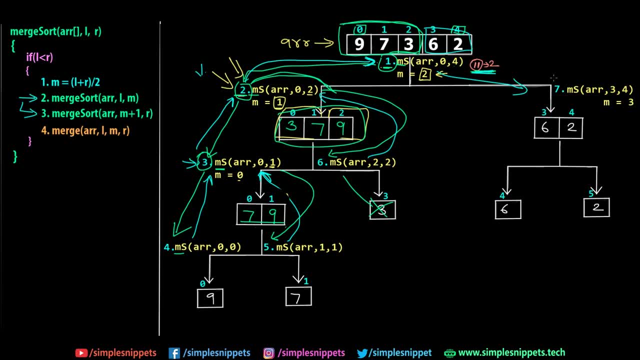 So now we have six and two. Let's see that. So this is how the seventh merge sort call will look like, And again, the first merge sort at this level will go pause at step number three. So let's do that. If you have a pen and paper, you can actually draw along with me for the best understanding. 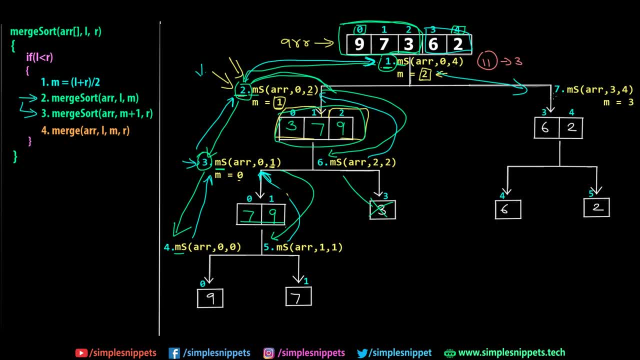 So merge sort number one is now paused at step number three and it has called a seventh merge sort. That's why it is paused. The seventh merge sort will be having the values of ARR three and four. So where do we get this three and four? 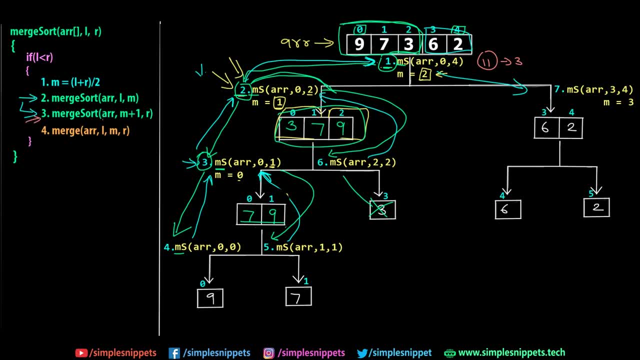 Because the first merge sort has called this Third step. What is the third step? You're passing array as it is, This array M plus one. What is M over here? At first level M is two, So two plus one is three. 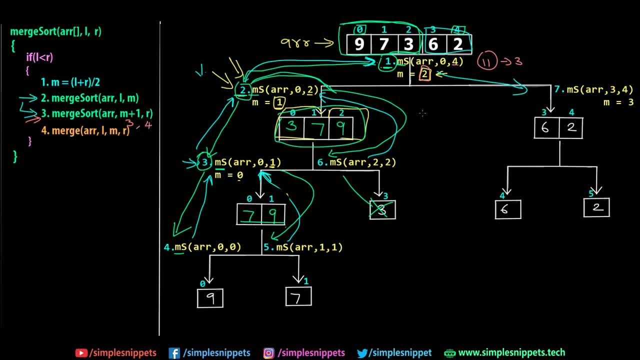 What is R over here? R is four, So four is passed as it is and hence the call three and four. Now over here, the midpoint is again calculated because we've passed three and four. Is three less than four? Yes, it is true. 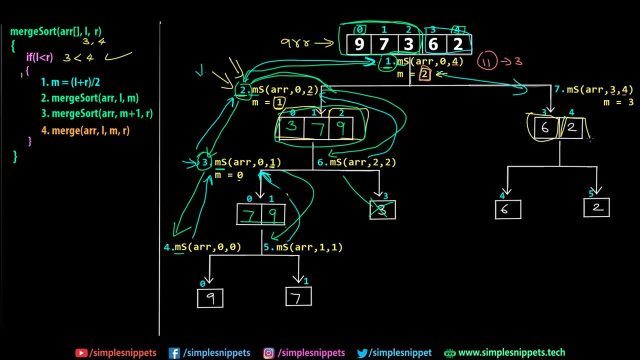 So again, division is going to happen. We have to split six and two into separate subarrays. Okay, So that's why we calculate midpoint. So the midpoint is given by L plus R by two. three plus four is seven. seven by two is: 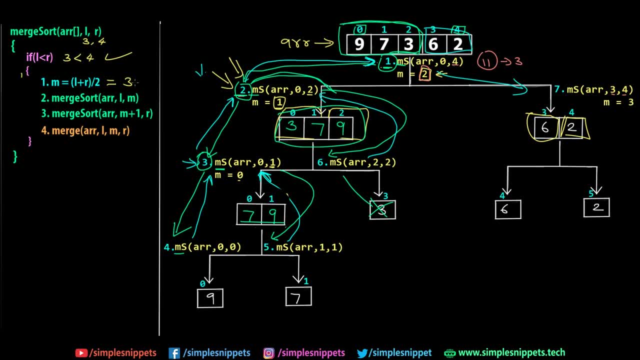 3.5, which is actually going to be three because we don't have an index with 3.5. So this is the midpoint itself. So that's how we're going to split it. We've splitted it. Now we will call merge sort, again on the left side, which is this side. 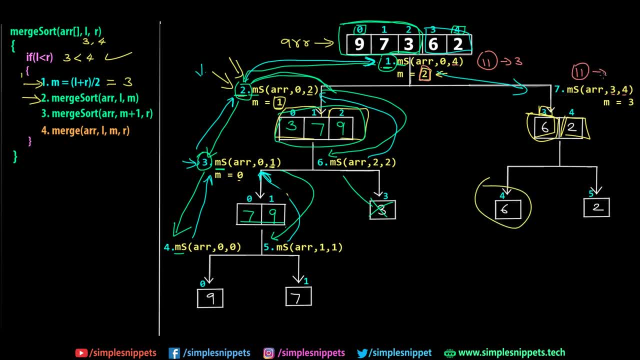 So again, seventh merge sort is going to go in pause state at step number two right. So at this state The seventh merge sort is paused and it has given a call to another merge sort, which is eighth merge sort, which looks something like this: 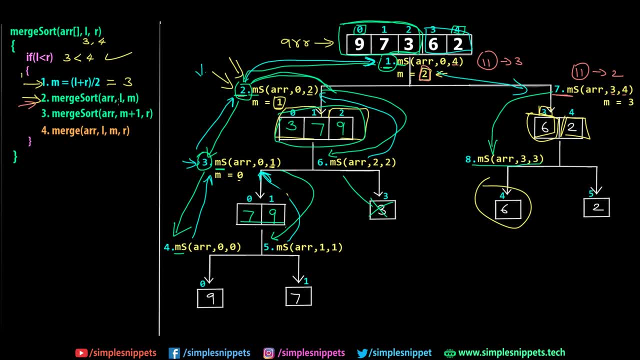 And over here we've passed array the left value. we've passed as it is. What was the left value over here? It is three. So we've passed it as it is in the array. but the right value that we've passed is the. 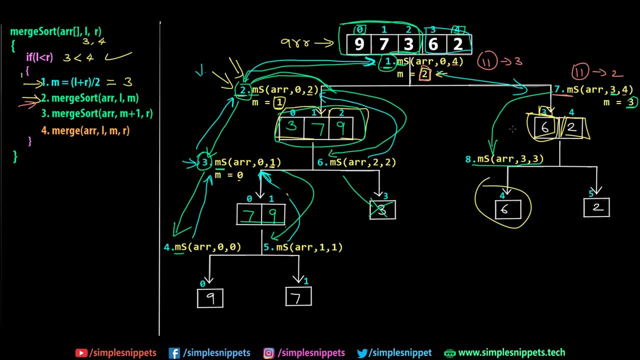 new midpoint that we calculated. What was the midpoint that we calculated? Three. So we've passed three comma three over here, right? So continuing or calling this merge sort again, we will pass three comma three over here. This time, three is not less than three and this entire if block will not be executed. 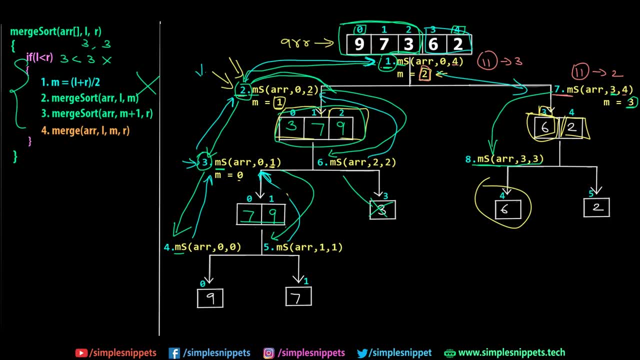 So that's why we've not calculated midpoint over here. We are left with only one single sub array element. So this merge sort will be done with the execution. It will go back to the calling function, which is the seventh merge sort. Seventh merge sort has been paused at step number two, right. 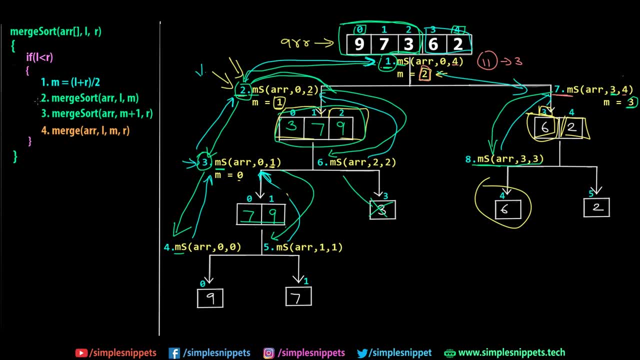 Now it will resume, So let's erase this. It was paused at step number two. It will move on to step number three. Now, step number three is another merge sort call for the right part. So we applied merge sort on the left part. 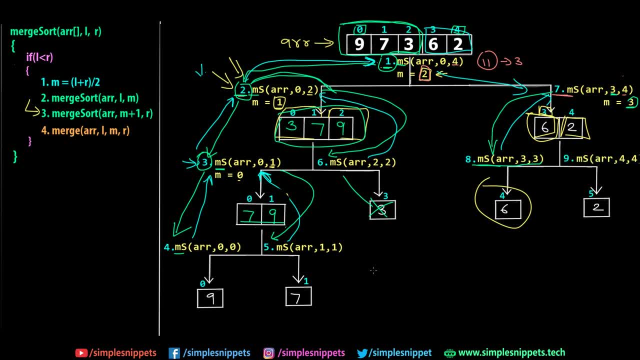 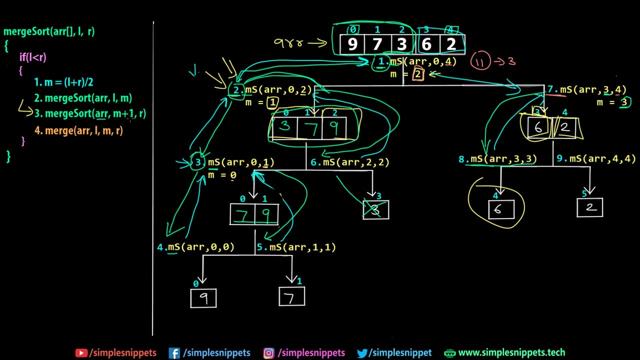 Now we have to apply merge sort on the right part. So this is how the merge sort call on the right part looks. We are passing ARR four and four because we are passing the same array. We are passing M plus one. M is three. 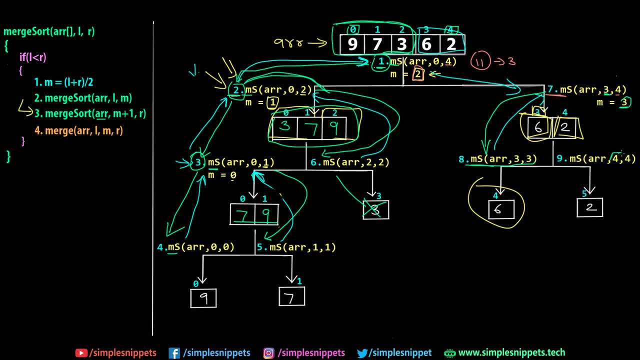 What is three plus one Four. So we will pass four. That's why the left index is passed as four and the right index is going to be as it is, which is four only. So four and four is passed. Obviously, when four and four is going to be passed, four comma four, four is not less. 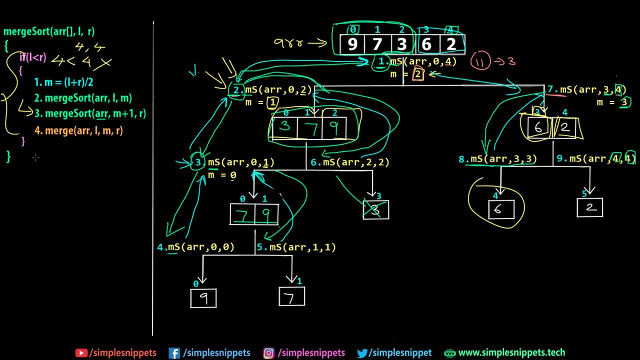 than four. This is wrong or this is false. So this entire block will not be executed. So the merge sort will return to the calling function over here, which is the seventh merge sort. Now, seventh merge sort was actually paused at step number three. 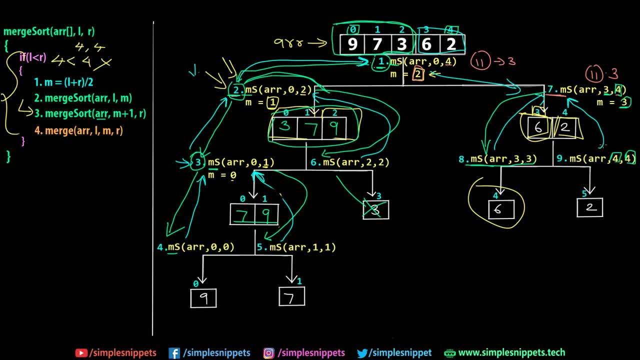 Since step number three is a merge sort call to the right array, which is actually done, it will resume. So just erase this And it will resume from step number three and it will move to step number four. Now, at step number four, what is happening? merging. 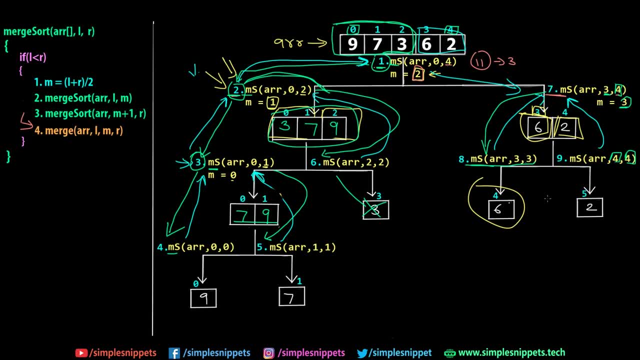 So at this level, what is the merging that has to happen? We have to merge six and two. So when we are going to merge them back we will compare. So that will happen in this merge function. As I mentioned, I will discuss this merge function in detail. 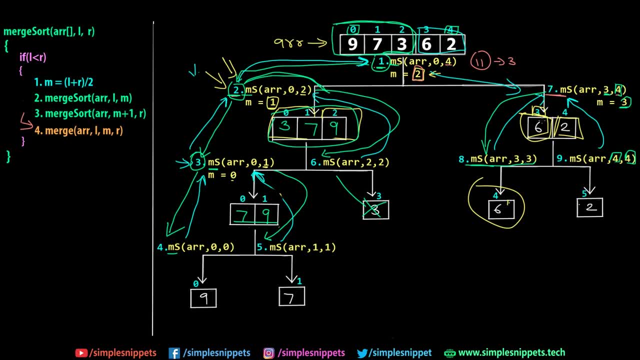 But what will happen? We will compare six with two, which is the smaller one, two. So two has to come over here and six has to come over here, So that swapping will happen over here, And now we will have two and six. 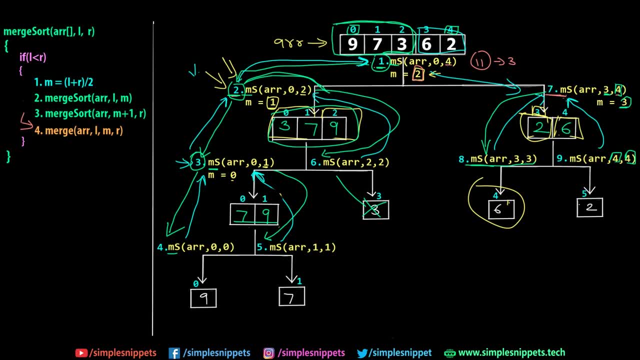 Okay, So this is the fourth step for the seventh merge sort call, And after this, obviously this entire merge sort will be done, which means this merge sort is also done. So who had called this merge sort? It was this one. You can see this arrow. 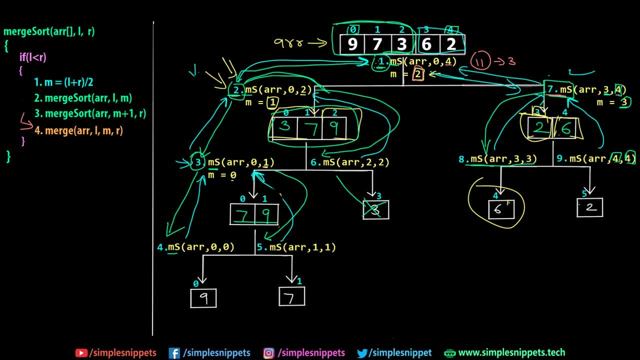 So now we will come back from seventh merge sort to the first merge sort, which had given it a recursive call. where was step number one? that is, where was the first merge sort? paused at step number three. What is step number three? Step number three is this merge sort call. 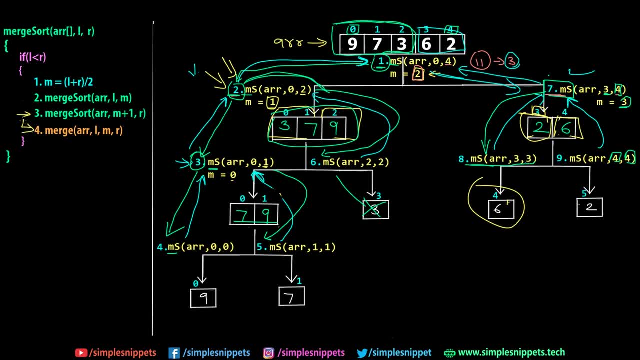 That is the rightmost merge sort. So now we will do the merge. And this is the last merge wherein you can see at the top level, Now we only have to merge three, seven, nine and two and six at this level, right. 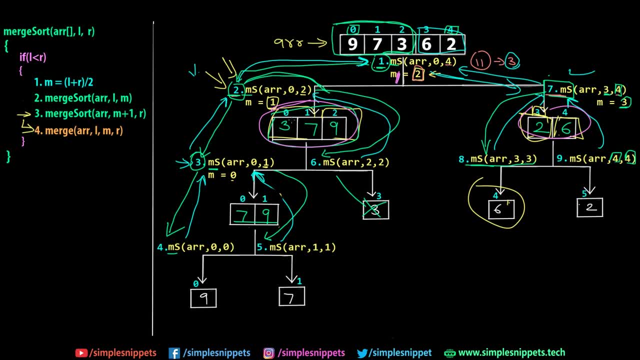 How will the merging happen? Again, comparisons will happen with three and two. which is smaller between three and two? two right. So let me just write it over here in between- somewhere I know things got a little cluttered. So comparison will happen between three and two. 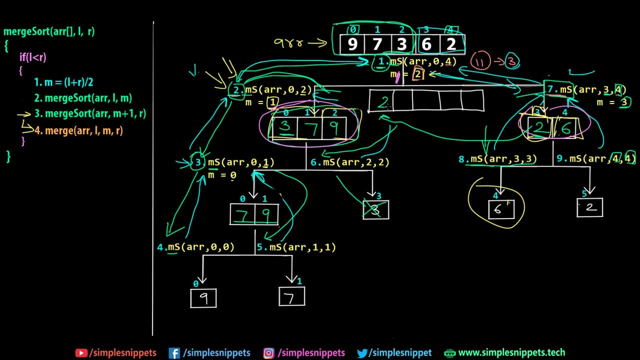 Which is the smaller one, two, So two will come in the first place. Okay, And this block will be eliminated. eliminated, or the iterator or the index that is keeping a track of this will be incremented. That will happen in merge function. 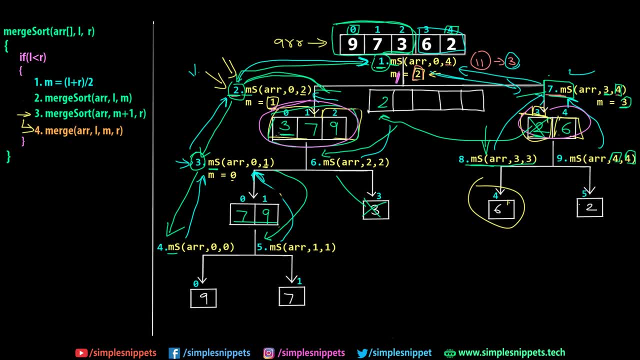 And I will explain to you in detail. The second comparison will again happen with three and six. which one is smaller, three. So three will come over here and this block will be eliminated, or the variable that is keeping a track of this index will be plus- plus. 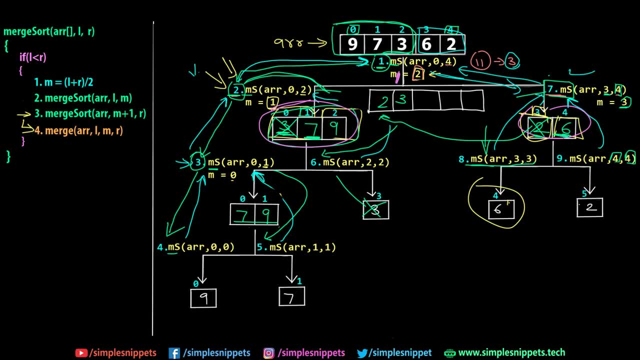 Incremented. So now comparison will happen between seven and six. which one is smaller, six. So six will come over here and this will be incremented. So, lastly, we are left with seven and nine, which is already sorted. So we will copy them as it is: seven and nine. 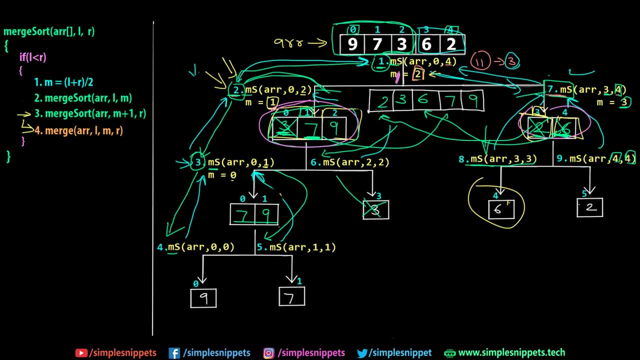 And there you go. You can see this is the final output we are getting in a separate area. We will store it in a temporary area and then transfer it back into our original area. So nine, seven, three, six, two, which is not sorted in any order, will be sorted in. 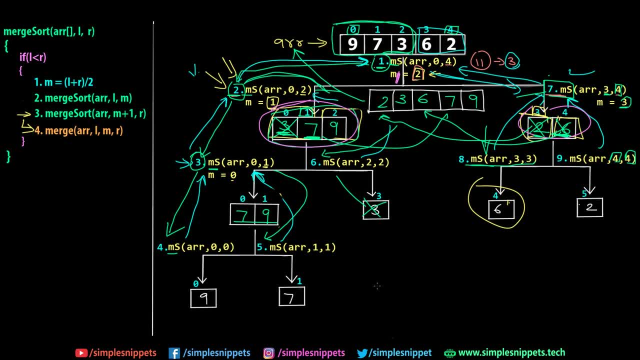 two, three, six, seven, nine In a ascending order. So this is the entire merge sort sorting algorithm, wherein we saw, step by step, how the recursion is going on, how the division is happening, how the merge sort is calling on itself, and 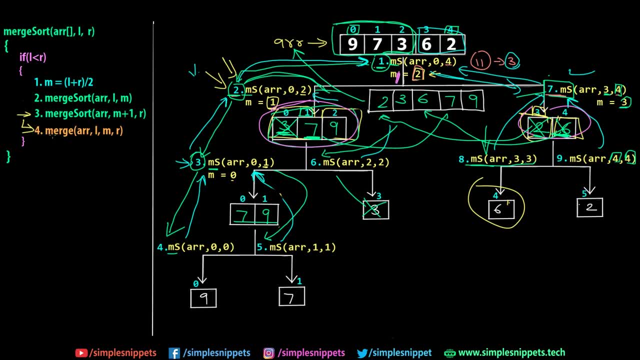 ultimately how the merge is happening. Now, one last thing that I have to explain over here is: how exactly is this merge happening? right, Because when we are coming or building back from the smaller subarrays- that is, nine and seven- some comparison has to happen. 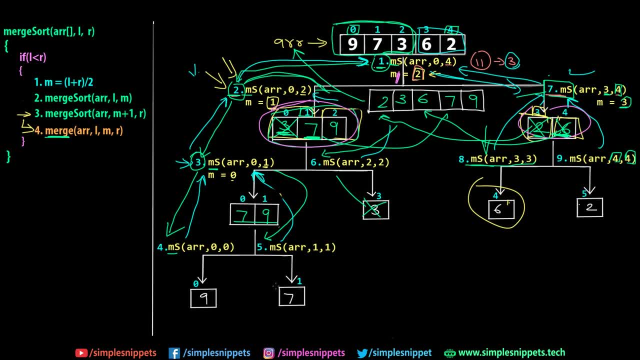 Some logic is supposed to be written which says that nine is greater than seven, So seven has to come first, right? So that algorithm or that logic is written in merge. So now let's see how this merge happens. Okay, Okay. 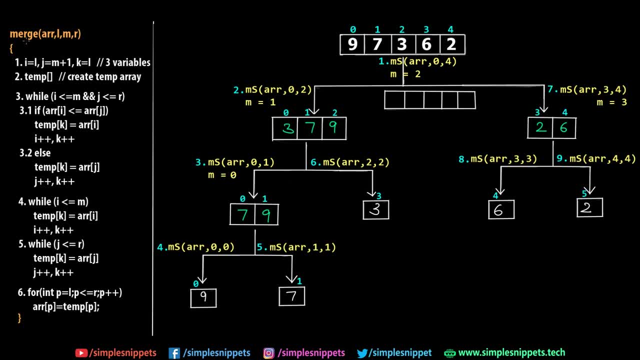 So, as you can see, on the left hand side, I've written the entire merge function. So what was looking as just a fourth step in the merge sort algorithm when we actually see what is exactly happening. So these all things happen and don't worry, this is not actually complex. 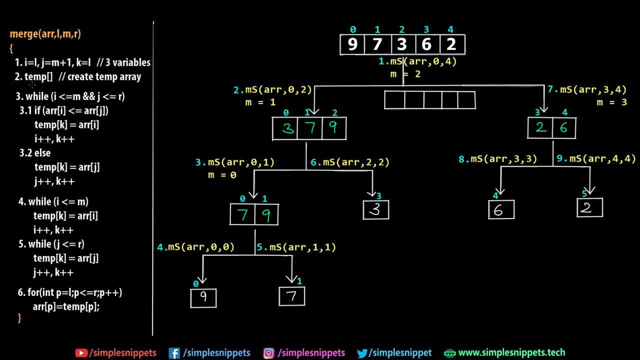 This is just a little lengthy, but it is very easy to understand. We will understand it step by step. So this is the complete merge function. Okay, This is the logic where the comparison happens, where the sorting happens and the merging happens. 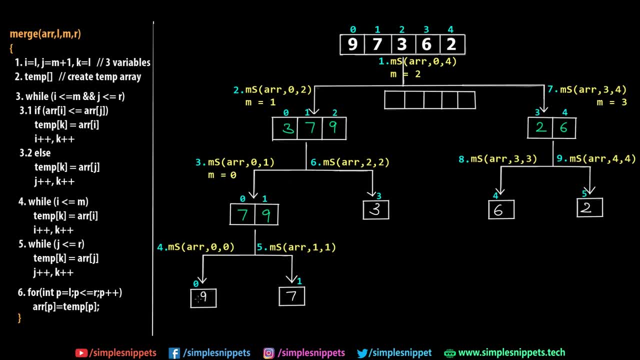 Okay, So on the right hand side, what I've modified is I've written the entire merge sort diagram as it is, And we're assuming that we've arrived at this step. that is, three, seven, nine and two, six, which means merging has happened at this step and merging has also happened at this step. 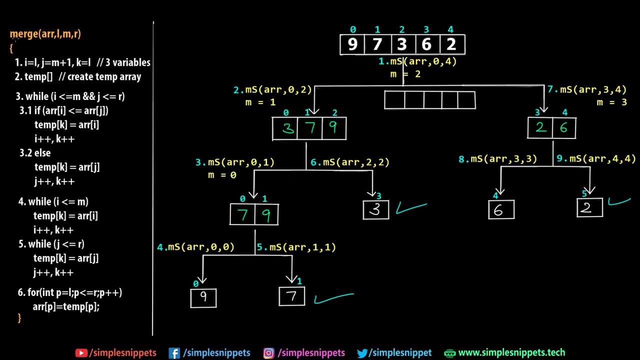 And now we are only left with one merging. So if I explain to you one merge function, obviously the same thing is going to apply at the smaller levels also, So I don't need to explain to you Over and over again, Otherwise it would be a waste of time. 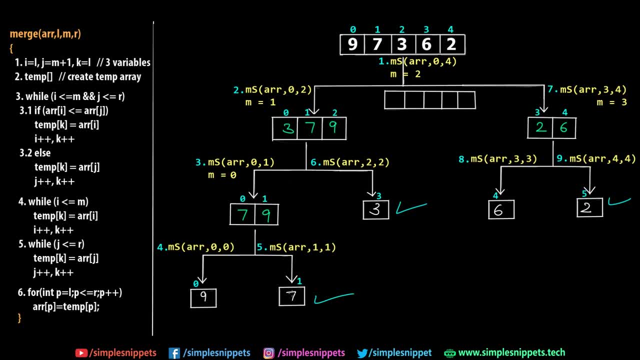 So if you just understand one time, it is the same thing that applies at every smaller step when we are doing the merging back. Okay, So when we are merging back from nine and seven to seven and nine, merge is called Again. when we are merging seven, nine and three, again merge is called. 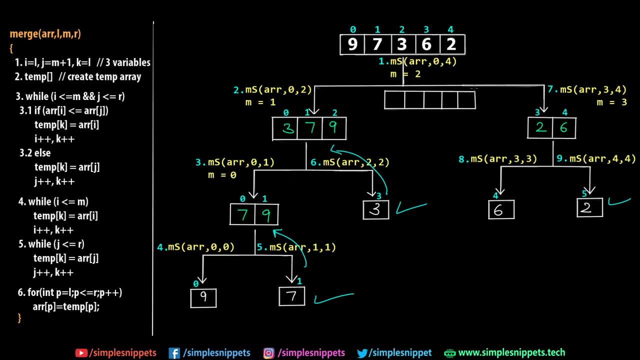 And then we are finally merging the two main subarrays into the final array. So again, merge is called. So if I explained to you for one time, everything applies the same for all the smaller merge calls, All right. So how do we merge three, seven, nine and two and six back together in a way that we 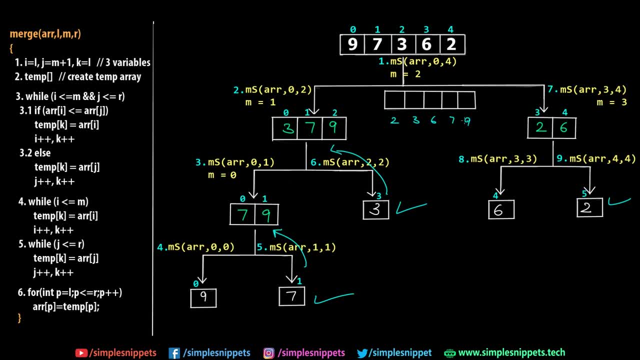 get the final result as two, three, six, seven, nine. We want a sorted array, right? So this is the result that we want to achieve. So we do this using a concept called two finger approach or two pointer approach. That's what it is called. 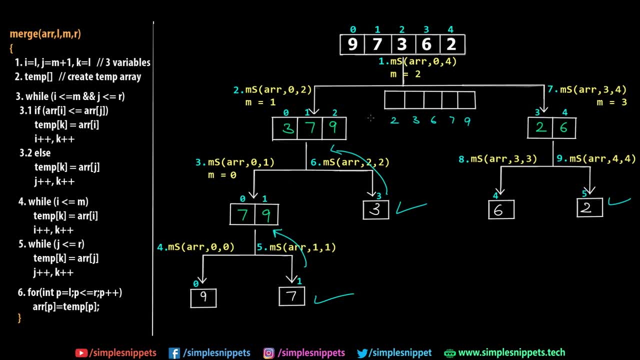 But what actually it means is we keep a track of pointers which actually keep a track of this index. So we keep a track off Yeah, Yeah, Yeah, Yeah, Yeah, Yeah Yeah. We keep a track off the left subarray and we keep a track of the index of the ride. so 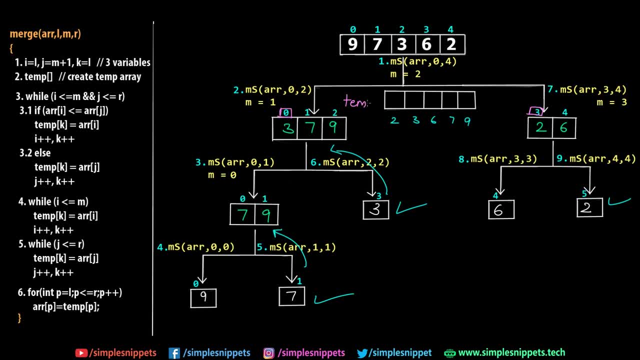 Barry, and we create a temporary array. So this is like a temporary array and obviously it will also have indexes, right? So let me just take it a little down. So obviously this temporary, I will also have indexes, so we keep a track off this index. 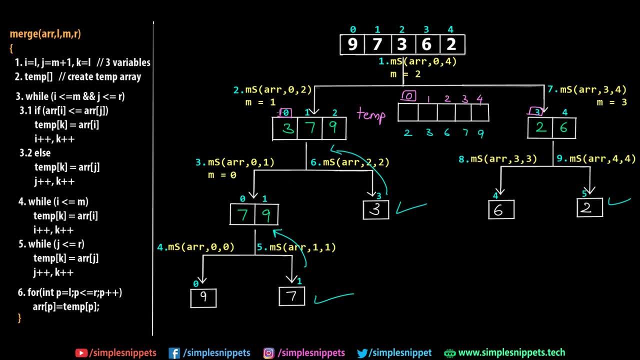 also. So we have three different variables which will keep a track off: the index of the left, serve up there, the index of the right side and the index of this temporary area. Okay Yeah, this merge algorithm or merge function, which is the fourth step of the MergeSort algorithm. 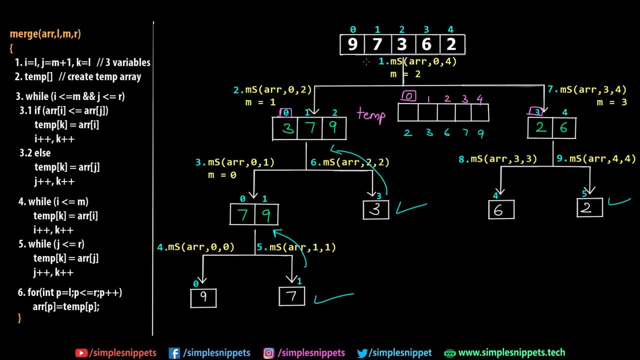 on these two subarrays. So when we do that, when we are at this level, when we are at this level, we have to merge this subarray and this subarray. right, That is this one and this one. So, at that level, what do we have the values of? We have the array, we 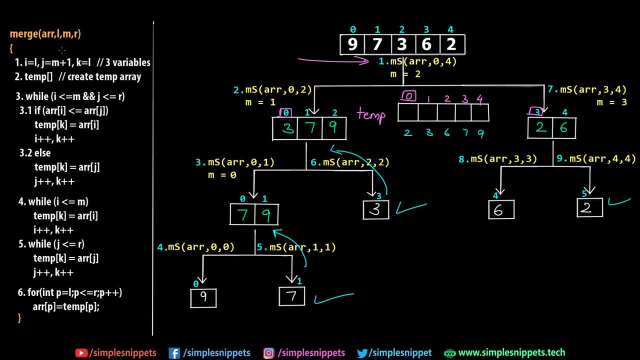 have 0, 4.. We also have the midpoint as 2.. In the merge call, what do we need? We need the array, we need the left, we need the midpoint, we need the right part or the right index. 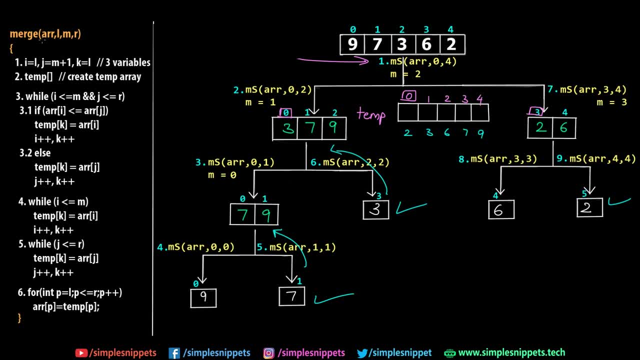 We have all of them over here, So we pass them as it is. We pass the array arr. Okay, We pass left index, which is 0. So at this level the left index is 0. Obviously, at the smaller levels the left index will remain the same. The right index will keep on changing. 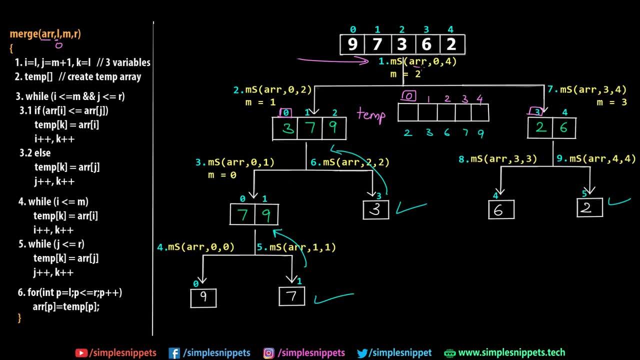 and on the right hand side, the left index will change. Okay, So at this level we have 0 and 4.. So we've passed 0, we've passed 4.. So let me actually write it down over here itself in a proper way. Okay, So we've written: L equals to 0. 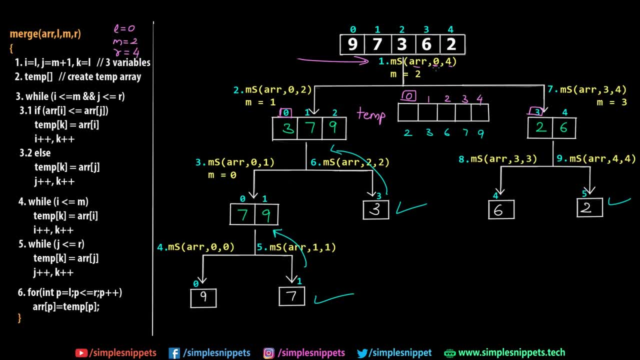 M equals to 2.. R equals to 4.. The left index is 0. coming from over here, The midpoint that we've calculated at this stage, at this level, is 2 and the right index is 4.. Okay, Now, as I mentioned, we're going to keep a track of the indexes of the left array, the right array. 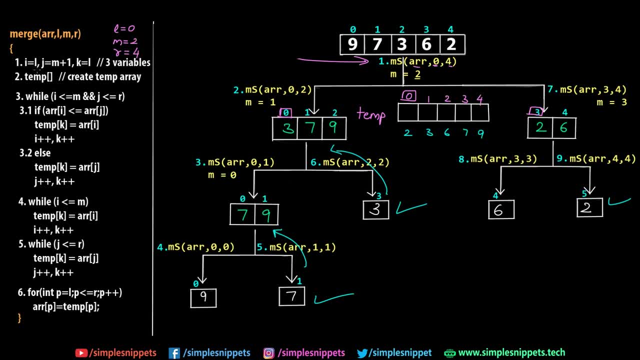 and the temporary array that we create. So we need three variables to keep a track of it. So these are the actual pointers. They're not really C plus plus pointers, Okay, So don't get confused that these are actual pointers. These are just variables which keep a track. 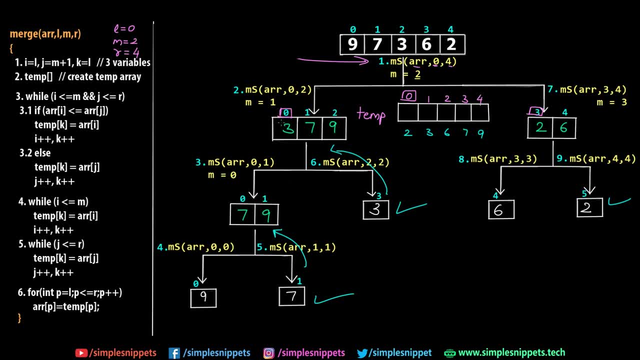 of these indexes And I'll tell you why we keep a track of these indexes. We'll need them for comparison purpose. So we say I equals to L. L is the leftmost index, right, So I is equal to L. So L is 0.. So I is going to be 0 for the first time. J equals to M J. 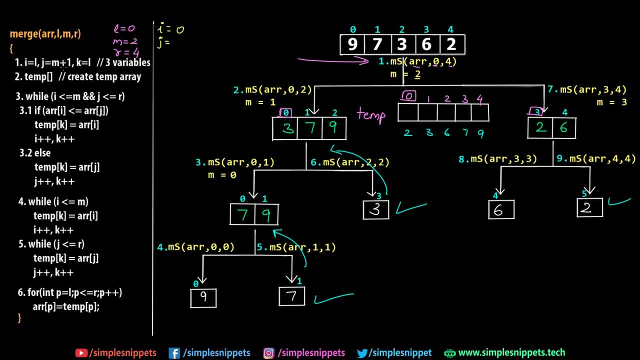 is equal to M plus 1.. It's not M, it's M plus 1.. What is M? Midpoint is 2.. We've calculated midpoint as 2.. So J becomes 2 plus 1, which is 3.. And K again becomes L, which is 0.. So 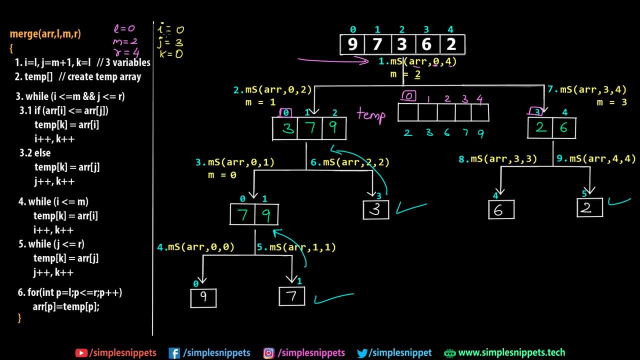 K becomes 0.. Okay, So these are the three pointers. Now, if you observe, I? equals to 0 is going to be the first index position for the left sub array. J equals to 3 is going to be the first index of the right sub array. So this is the right and this is the left. 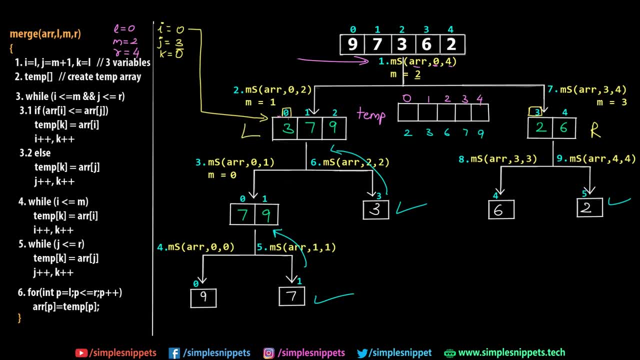 Okay. so we've got I pointing to the very first index position of the left sub array. We've got J pointing to the very first index of the right sub array. So what is this K doing? So K is going to be pointing to the temporary array. So K is this. I is going 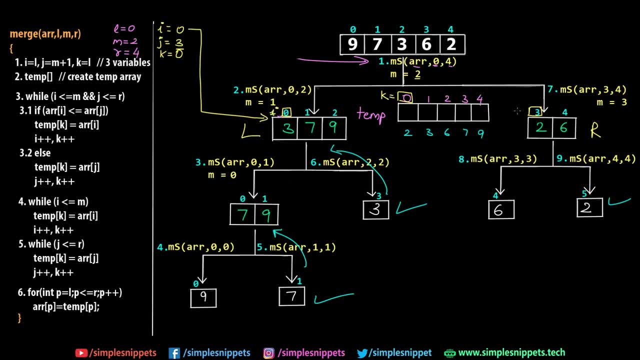 to be this. I know it is a little cluttered, but I hope you are getting it, And J is going to be equal to this. So this is how we initialize things at step number one. Step number two: obviously we're going to create the temporary array And you can create temporary array. 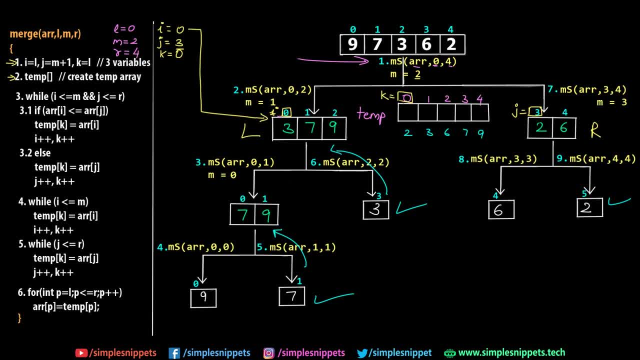 over here also at the first step, But K is going to be keeping a track of this temporary array. Okay, we create a temporary array. The third step is we are using a while loop. Now we want to check which value is smaller in either of the array. So what we are checking. 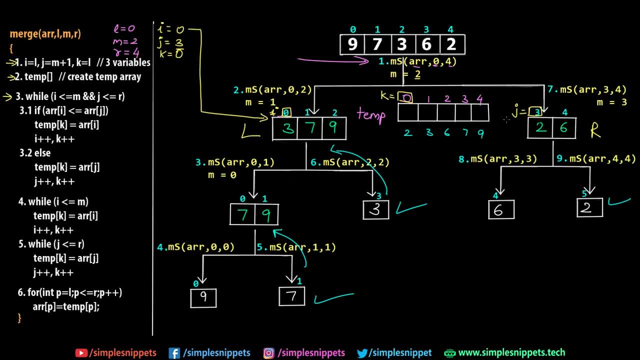 we are checking the first element in the left sub array with the first element in the right sub array And, depending upon which one is smaller, we're going to transfer it in the temporary array right. So we need a condition which will iterate to 379 and 216.. Now you 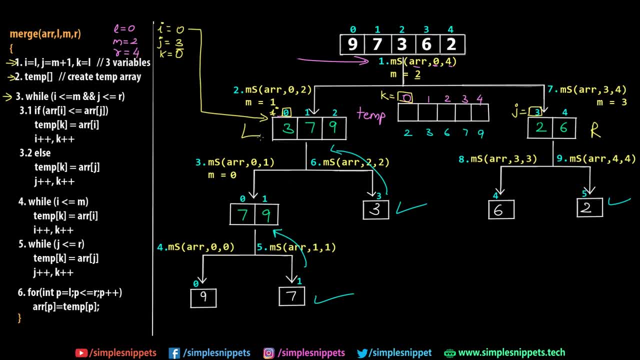 can see that this is odd setting, right, odd setup, which means that left sub array has one element extra compared to the right sub array. So we are going to create a temporary array. So it is highly possible that either of the one sub array gets exhausted first. 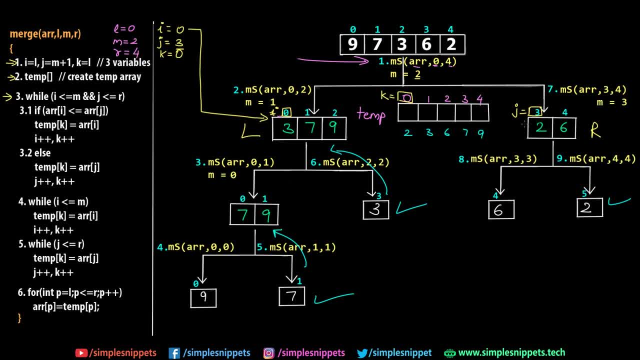 which means, let's say, if the right sub array gets exhausted first, all the elements in the left can be directly copied as it is, and vice versa. Now, if it doesn't make sense, let's just actually apply this. So the condition is: while I is less than equal to m, I is the 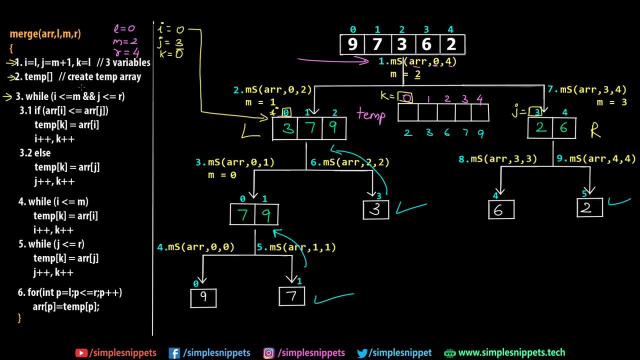 iterator for left sub array and I over here is zero. m is actually equal to two. you can see, m is equal to two. So for the left sub array, we are going to create a temporary array. So we are going to create a temporary array. So, for the left sub array, what are the valid indexes? zero. 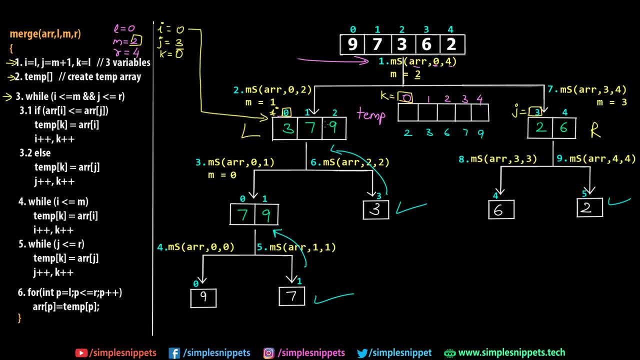 one and two. you cannot go to three right, Because left sub array is only comprising of three elements. So that's why this first condition is to be in the left sub array limits, that is, the index limits. So this condition will restrict the while loop to iterate only. 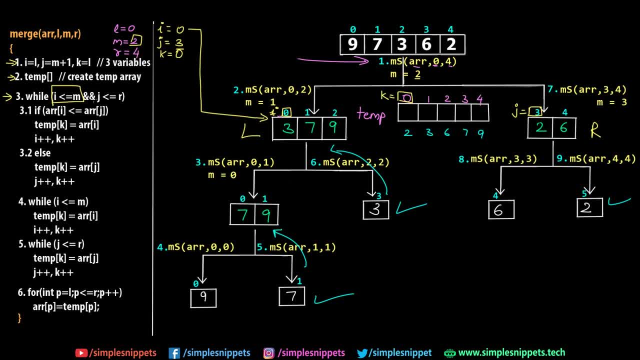 in the left sub part. But then we also have a and clause which says: and j less than equal to r. So what is j? j is three, which is the starting point of the right sub array. So j zero is the starting point of the right sub array, And j can iterate between three. 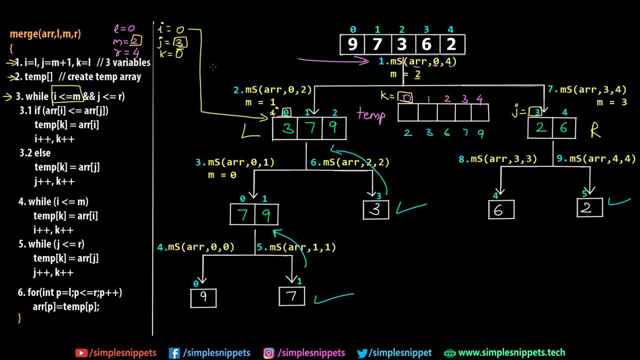 and four. only these are the two valid indexes for the right sub array. What is the value? of our r is four, So that's why we are keeping a track of both the index ranges using this condition. So there is a and clause in between, because it is highly likely or highly possible. 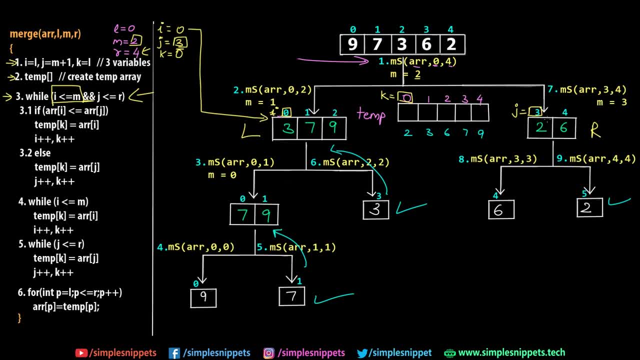 that one array will get over first. that is, we will transfer all the elements of one array into the temporary array And then we cannot go further in that array. right? We cannot array right, we cannot make any further comparisons. so that's why this while loop or condition. 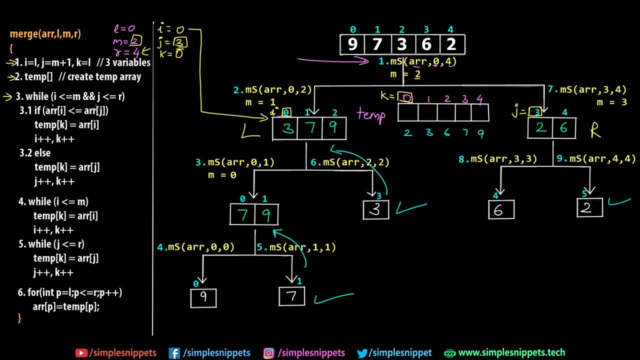 is used. you'll understand more as we actually dry run this. so let's dry run it. so, initially, obviously i is 0 and 0 is obviously less than m. m is 2, correct? so i is 0, m is 2. what is j? j is 3 and what is r? r is 4. so this is less. this is less. both conditions are true because 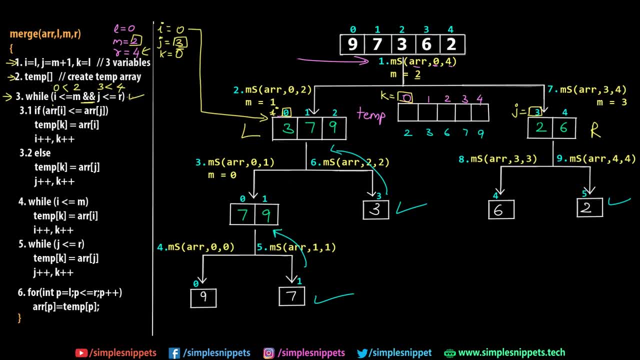 there is a and clause. both have to be true and since both of them are true, we go inside this while loop. so this is step number three. inside the while loop, we have step number 3.1 and 3.2. now this is where the actual comparison is happening. okay, so what is this comparison? 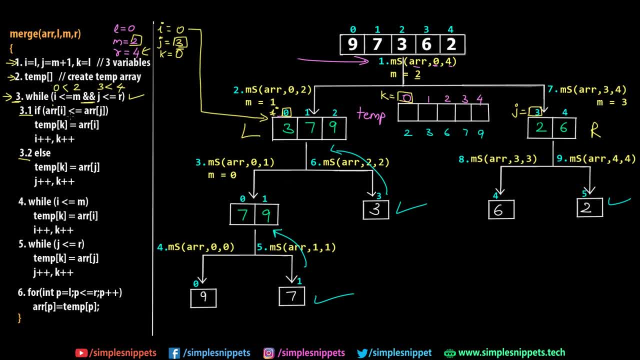 happening. so, for the first time, we are checking if arr of i is less than equal to arr of j. what is i? i is 0, so arr of i is arr of 0, which means this element is 3 less than m. m is less than equal to arr of j. what is j? j is 3. what is arr of j? this element is 3 less. 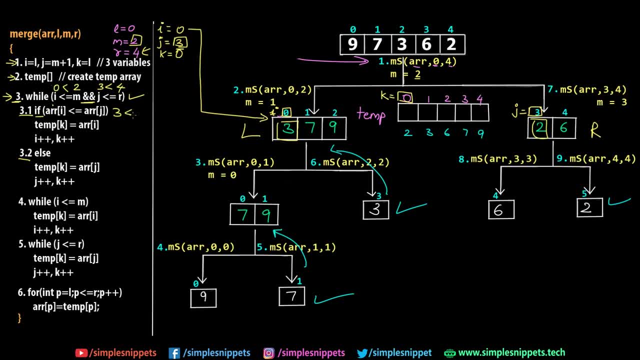 than 2. we are checking if over here is 3 less than 2. over here obviously it is not less. 3 is not less than true. so the if block is not executed right. so these two steps will not be executed. we will go to the else part. in the else part, what we do since we've now 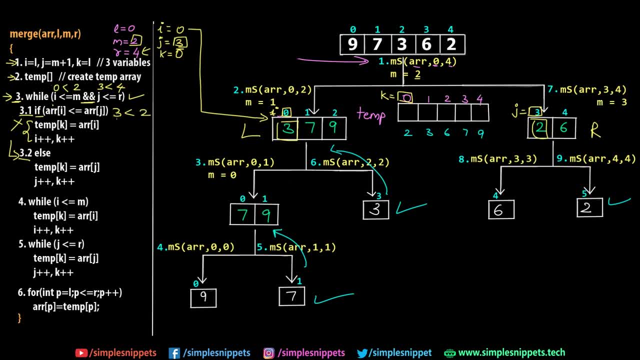 achieved the fact that 3 is not less than 2. obviously 2 is less than 3. so we will say: temp of k equals to arr of j. so we've determined that from the left array and the right array 3 is greater than 2, which means 2 is smaller. 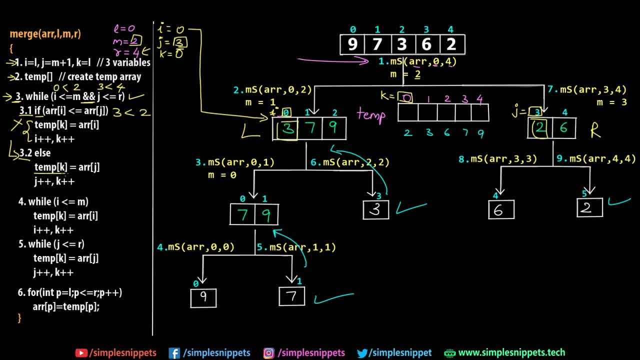 so 2 has to come first in the temporary array. so we are saying temporary array of k. now k is 0. we started k with 0, so temp of 0, that is, at this location we want arr of j, which is 2, so 2 will be transferred over here. so i'll write 2 over here now. look at this next. 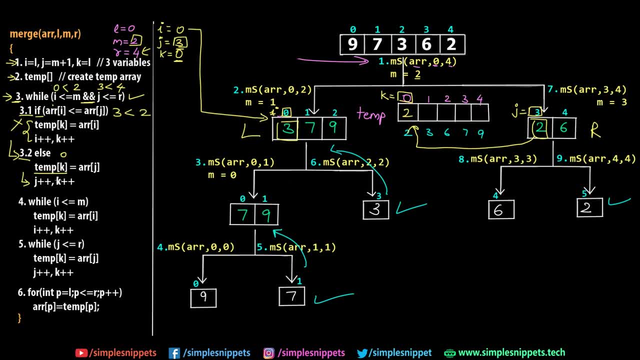 step which says j plus plus and k plus plus. so what did we do? over here? now k is less than 2, so this can now be converted over here, so longer than 1 from x 6 to 22.. this is the two steps, that is, if and else inside the while loop. So once we complete, 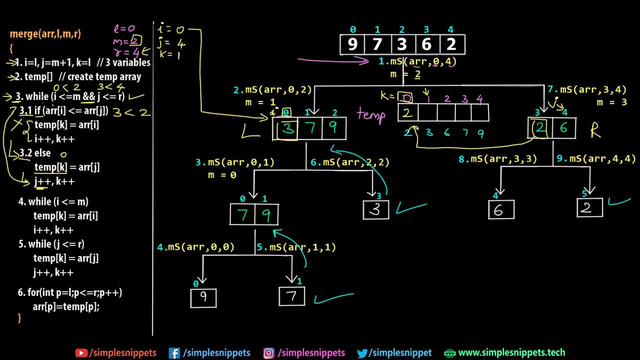 the else part, we will again go to the start of the while loop, obviously because while loop will keep on executing till the inner condition is true. So let's again evaluate the inner condition now. So again, second time we are checking: is i less than equal to m? 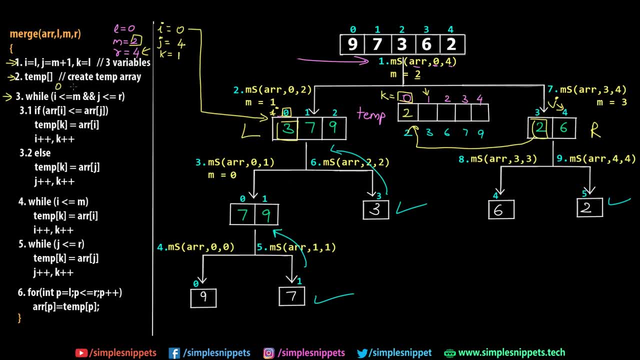 What is i? i is 0.. What is m? m is as it is. m and l and r are not going to change. The only thing that are changing are the individual variables that are used to iterate through all the indexes, right? So m is going to be the same. m is actually going to be 2 only. 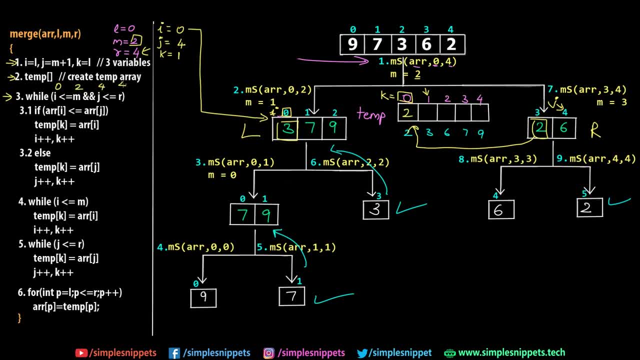 What is j, j has now become 4.. What is r, r, is also 4.. Now let's see if the conditions- both the conditions- are true. Is 0 less than 2?? Yes, it is. So this condition is true. Let's. 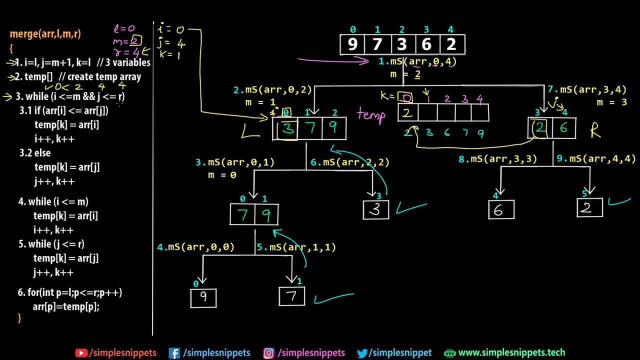 see the second condition. What is the second condition? and and j less than equal to r. So 4 is not less than 4, but it is equal to 4.. So this also condition is true right, because it has to be less than or equal to, So this: 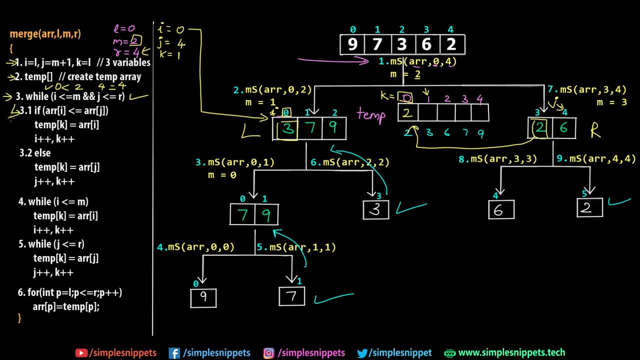 two conditions. both, again, are true. and now we again go inside the while loop. Now again a comparison is made if arr of i is less than equal to arr of j. So now what we are comparing? we are comparing arr of i. What is i? i is 0.. So arr of 0 is 3, right? So we are again. 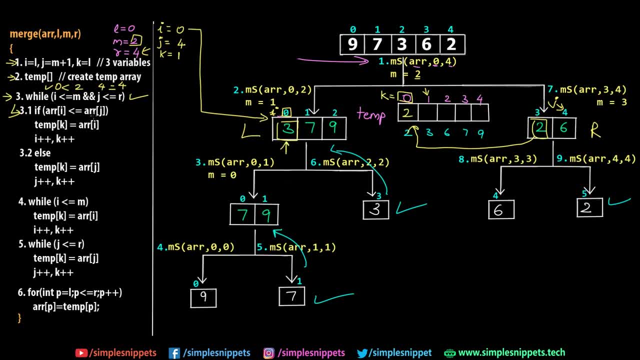 over here. only for the left sub array For arr of j, j has become now 4.. So j is pointing to this location now because this is already transferred. So now we are comparing between 3 and 6.. So you can see there is a pattern going on. there is a comparison now. 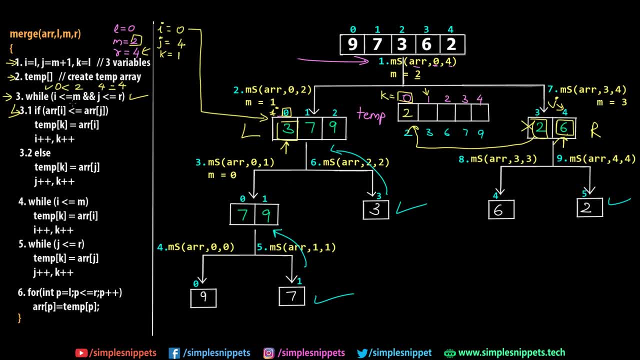 So now 3 is compared with 6.. Now obviously arr, which is 3, is less than arr. arr, this time, is 6.. So 3 is less than 6.. So that's why now this, if block will be executed: 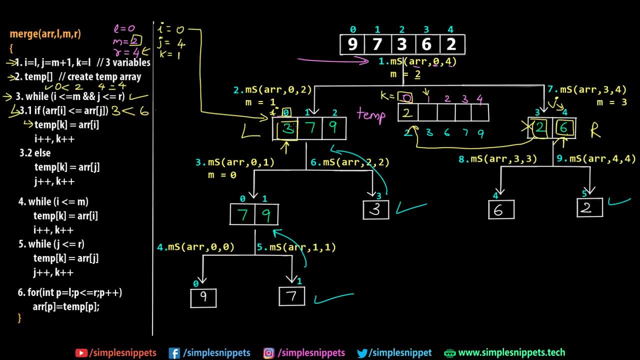 And inside this now we are saying temp is equal to arr. So since the element in the left array is smaller, we want that first to go in the temp array. So now 3 will be transferred over here. So temp, what is k? 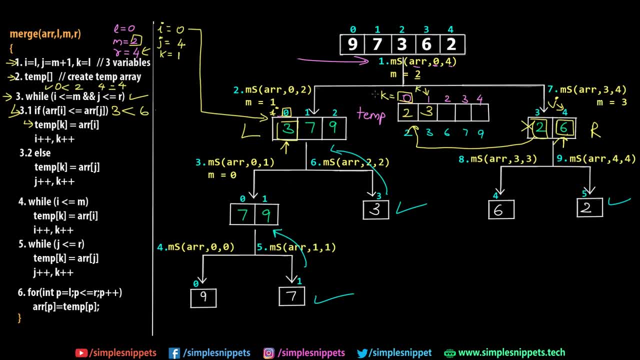 k is 1.. We are at this location. k was pointing over here and not at 0th location, So 3 will be going over here. Now we say i++ instead of j++. that we are doing in, else we are doing i++. 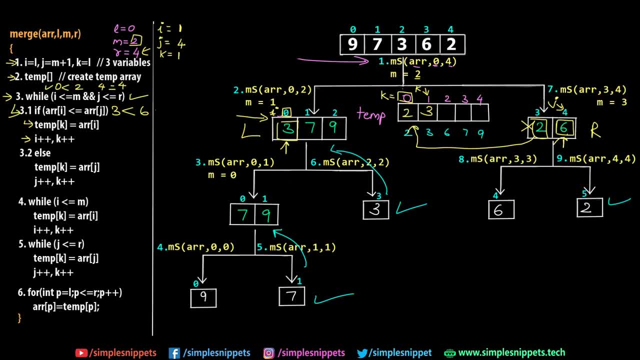 So now i becomes 1 over here, and again we increment the k because the second position is occupied, So k will now point to 1.. So k becomes 2. Now, since if block is executed, the else will not be executed, Either if will execute or else will execute. 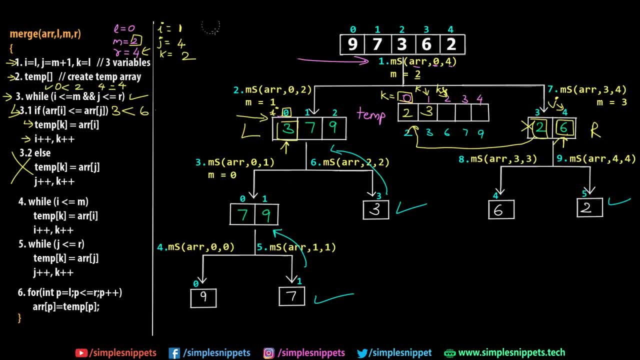 So now i has become 1.. So i will not point to this first location. I will point to this location: i has become 1.. So you can see the first two are done. Now we have left with 7 and 9 in the left array and 6 in the right array. 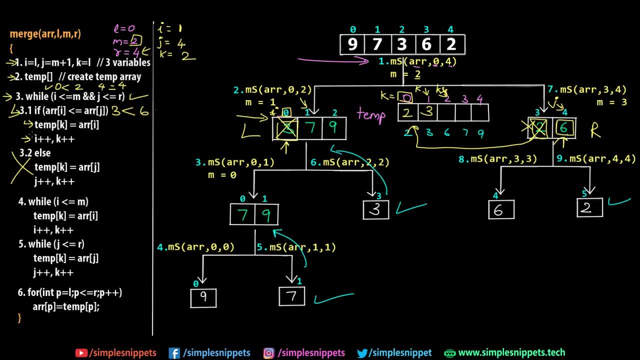 So now let's see what is happening. So we come at the end of the while loop, Because if is executed, else will not execute Again. we will come at the start to check the while condition. So, according to the while condition, what is the condition? 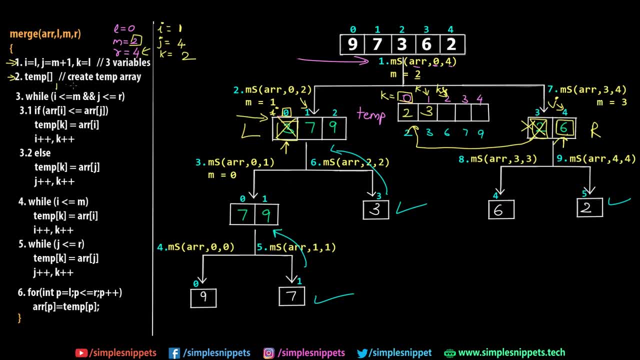 Is i less than equal to m? i is become 1.. m is obviously going to be 2 only, So 1 is less than equal to 2.. This is true. What is j? j has become 4.. 4 is less than equal to 4 only because r is also 4.. 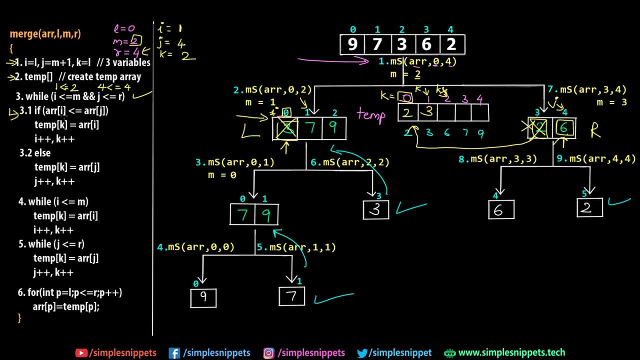 Again. it is true. So we will go again inside Again. a checking is done. Error of i. What is error of i? Error of 1.. Error of 1 is 7.. Is 7 less than or equal to error of j? 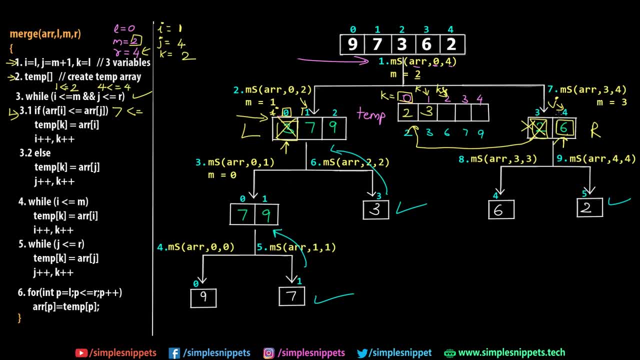 What is error of j? j is 4.. So error of j is 6.. Is 7 less than equal to 6?? No, 7 is not less than equal to 6.. 7 is greater than 6, right. 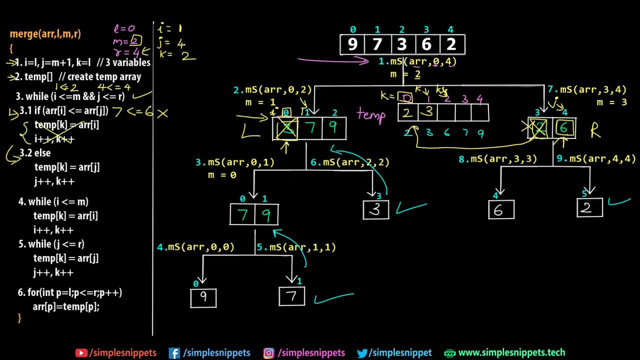 So if block will not be executed we will go to else block In the else block. what we've determined is 6 is smaller than 7. So we want 6 first. So 6 will be transferred over here We will say: temp of k equals to error of j. 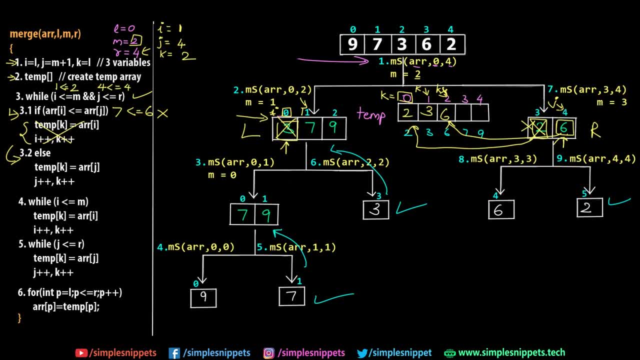 Because we want the value In the right subarray, that is, error of j, to go in the temporary array first. So 2, 3, 6 is happened over here. We are saying j++ and we are saying k++, So j will be incremented to 5 and k will be incremented to 3,, 5 and 3.. 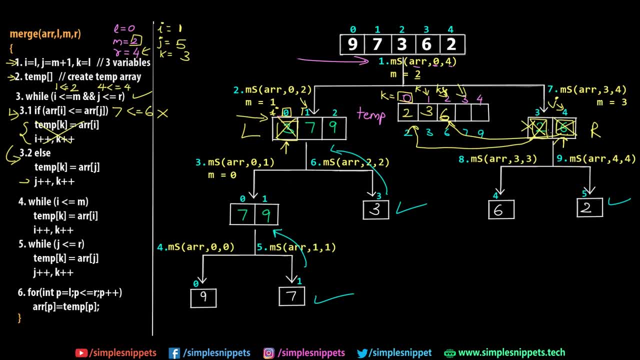 So now k will be pointing over here and j has completely exhausted. j has become 5.. Okay, So else block is done. We will come at the end of the while loop again. go at the start to check the while loop conditions. 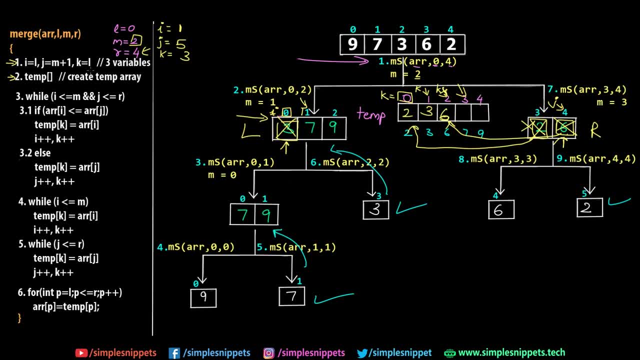 Now let's check the conditions. So now, if you compare, i is obviously 1,. 1 is less than equal to m, which is 2.. Now j has become 5.. Now, 5 is not less than equal to r, which is 4, 5 is obviously greater than 4.. 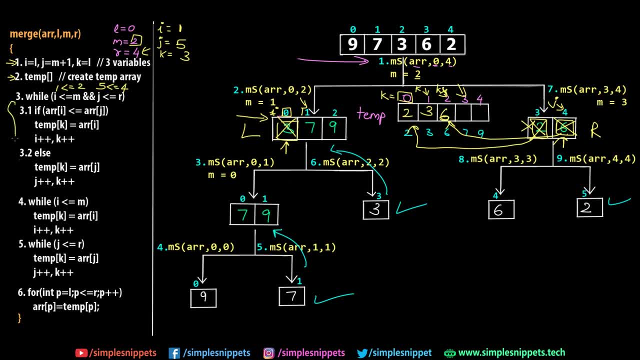 So now we have completely exited out of this step, number 3.. This entire while loop will stop executing and we come on the fourth and fifth step. So, since we've exited this while loop, if you observe, right now in the temporary array we still have two elements to be filled. 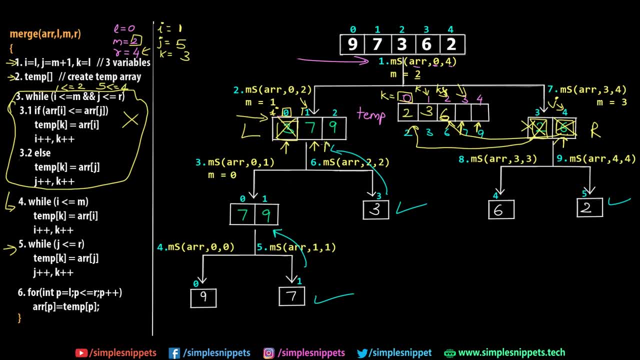 And both of them are only from the left array. right Because the right array elements are already in place in the temporary array, which means that this right array is exhausted. So you can see that when this while loop stops executing, we are still left with two elements. 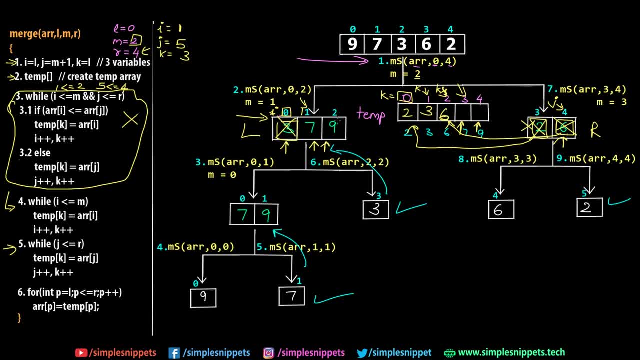 but both of them are from the left array. So that's why what we can do, we know that 7 and 9 are already sorted because when we were merging, when we are calling merge function at this location also, The same merge function is already sorted. 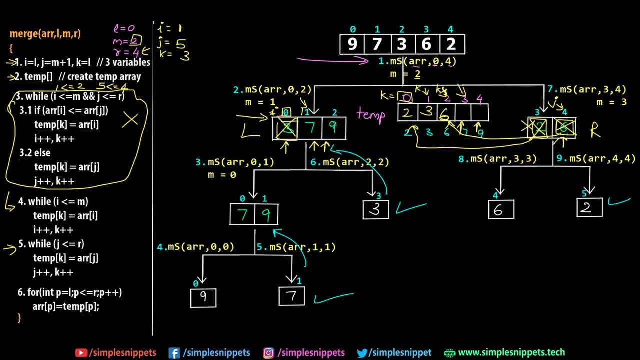 The same merging was happening and ultimately we resulted in 3,, 7,, 9.. So this is already sorted, So we can directly transfer them, as it is right. We know that, But when will we know that? when we actually exit this while loop and when we are still? 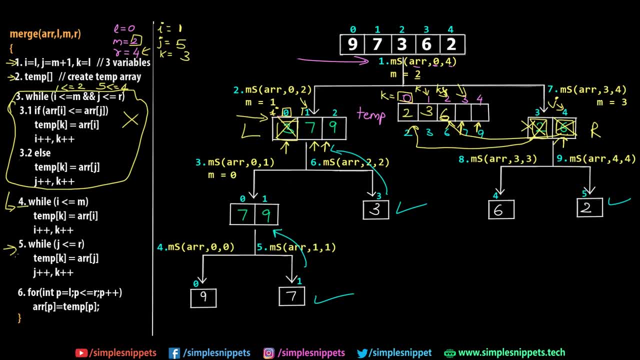 left out with some elements. So now the fourth and fifth while loop are only checking whether there are some elements left in left array or right array, And if any one of the array is exhausted first, the second array elements can be directly copied as it is, because they are already sorted. 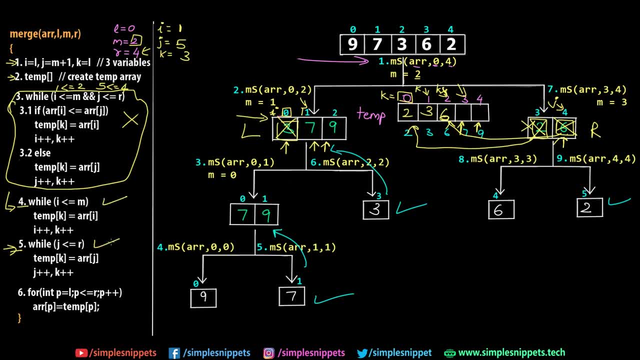 Okay, So that's the logic for this while loop and this while loop. Now, any one of this while loop will only run because one is already exhausted. One, one part or one sub array is already exhausted. So let's see if this while loop runs. what is the condition over here? is I less than? 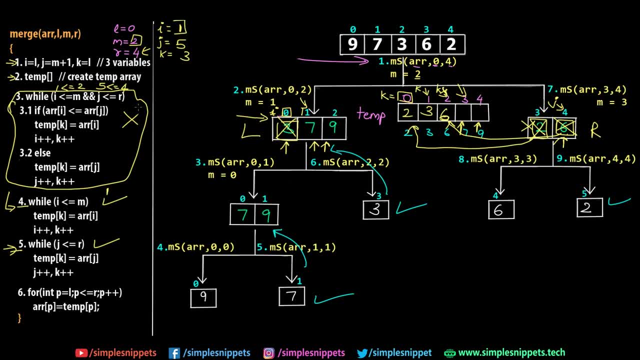 equal to M. I is one. Okay, What is M? M is two, which means this while loop will execute. this condition is true, And this determines that elements from the left array are left out, And since we know that they are already sorted, seven and nine is already sorted, right. 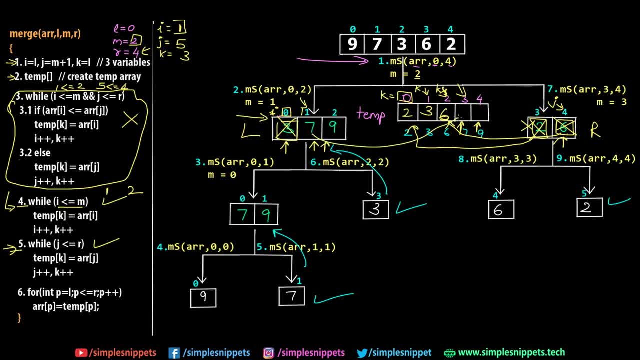 Seven comes first, nine comes next. We can directly copy seven over here and we can directly copy nine over here. So that's why you can directly say: temp of K equals to ARR of. I thread this step. What is I? I is pointing to one. 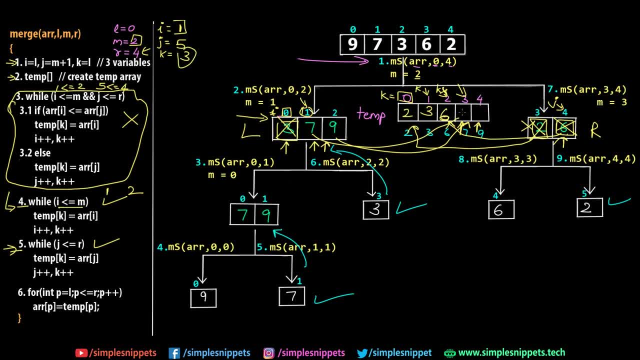 So temp of K. what is temp K? K is pointing to three, third location. So seven is directly transferred over here. I plus plus happens, and K plus plus happens, I becomes two, K becomes four. So K points to the last element. 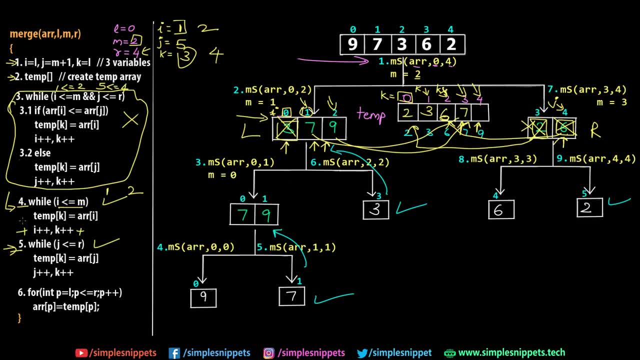 I points to two, which is this. So second time I becomes two. Is two less than equal to two? Yes, it is equal to two. So this again, while loop will execute and nine will be transferred over. here When we come on the step number five, we say: while J less than equal to R, J was become 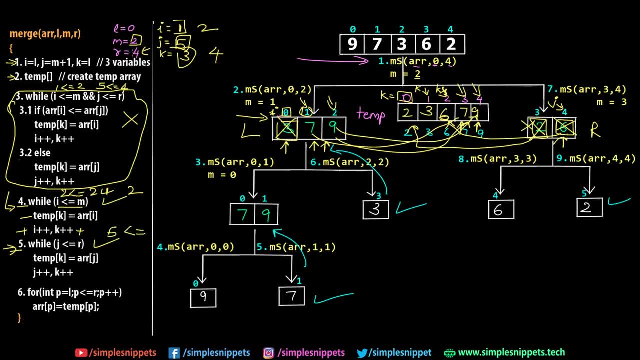 five over here, You can see, is five less than equal to the right value, which is for no. So this while loop will obviously not execute. And, anyways, we know that we've exhausted the values from the right sub array. We've already transferred them to the temporary array. 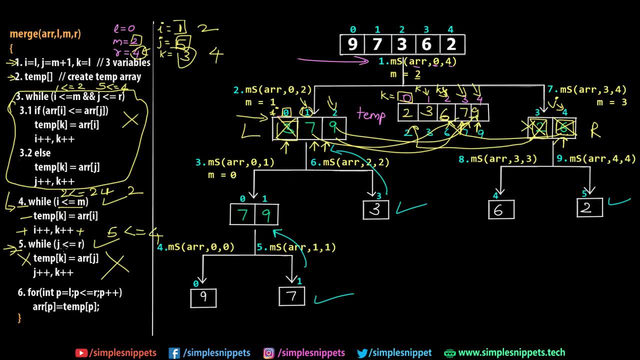 So no point in executing this while loop. So that's why this while loop will not execute. Now one last thing is left. If you observe two, three, six, seven, nine, we've already got the sorted temporary array, but this is stored in a temporary array in temp. 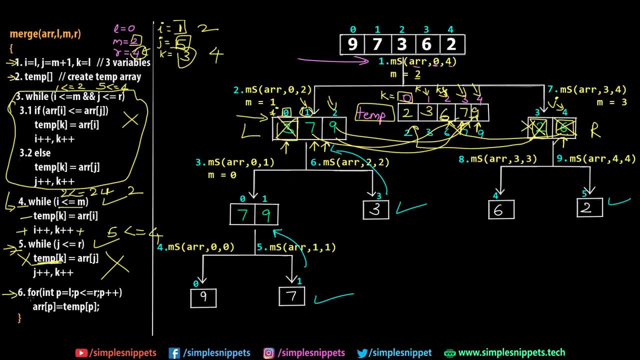 So the sixth step is where we use a for loop, basic for loop, to iterate through zero to four. That's the condition you can see in: P equals to L. what is L? L is zero. P is less than equal to R, which is four. 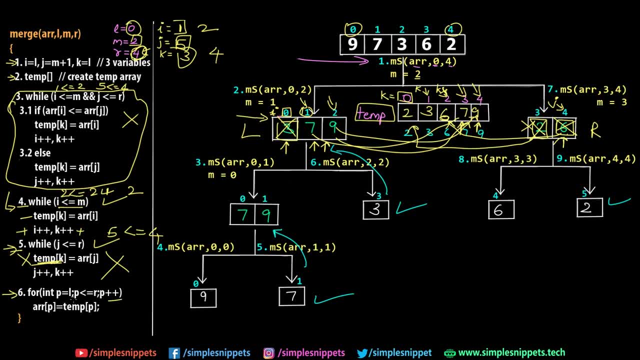 So zero to four, We are iterating from zero to four and we say P plus, plus and we are just copying all the elements from the temp, That is, this array- two, three, six, nine, as it is, into our original array, which is ARR. 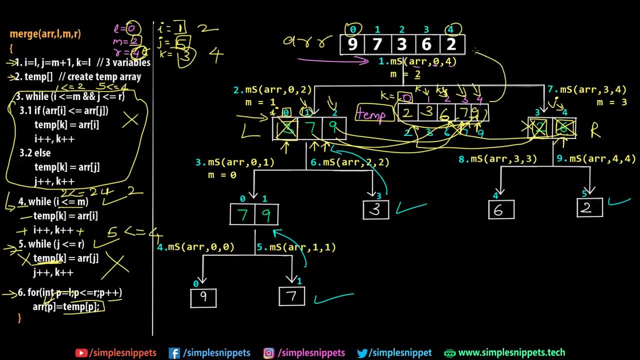 which is nine, seven, three, six, two, which is unsorted. So when we copy everything over here, finally we are left out with two, three, six, seven, nine, and this is the final array, which is sorted in ascending order. 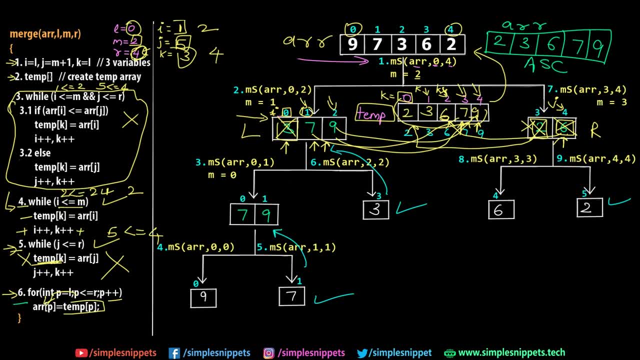 So, yeah, this is where the merge will stop and this merge happens at every step. Okay, So I explained to you: Merge This two levels. Now merging will happen at this level also. merging will happen at this level also because these two will be merged back over here. 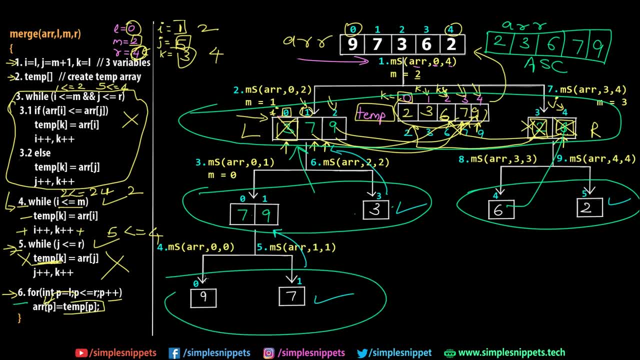 These two subarrays will be merged over here and merging will happen at this level also. These two will happen over here Now. same logic will be used. So if you want, you can pause the video. You can dry run this merge function for these smaller subarrays also by going step by step. 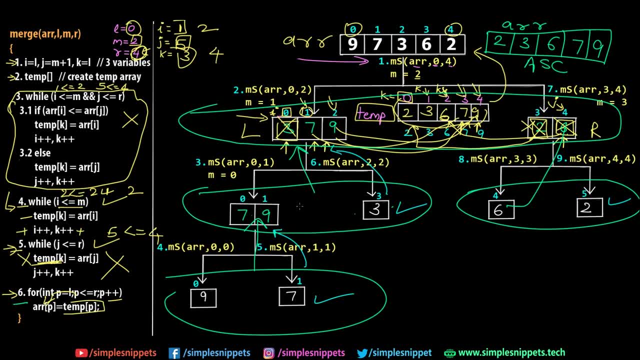 through these steps you'll get the same results, but this is how the entire merge sort sorting algorithm works And also specifically works. So I hope you've got a very detailed idea about how the merge sort works by dividing, then by recursively calling merge sort on individual subarrays. 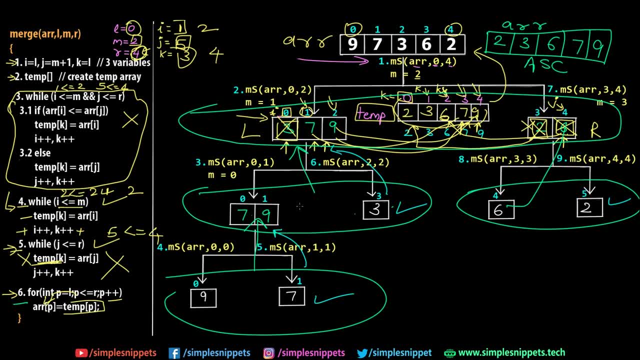 And then, ultimately, when we have only one single subarray element left, we call the merge function to merge everything back together. So yeah, this was the entire merge sort sorting algorithm. I know it got a little intense, It got a little serious and very heavy, but if you want, you can watch this video again. 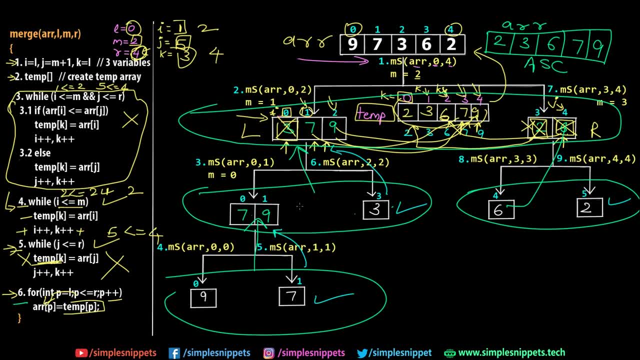 probably at a slow speed. If you want, go step by step, take a pen and paper and debug these algorithmic steps yourself. Keep a note of all the- you know- values, of all the variables at every step, so that you understand what exactly is happening.